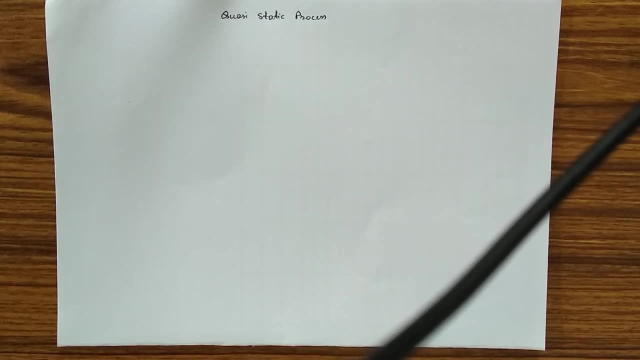 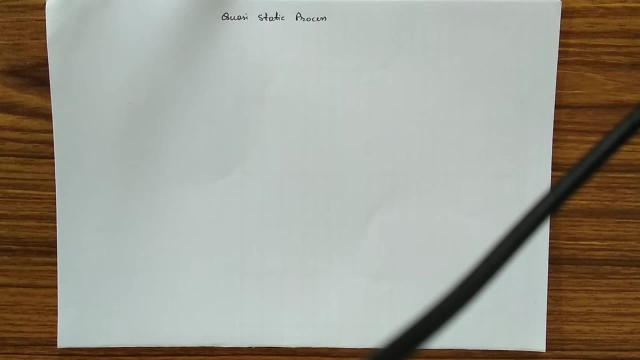 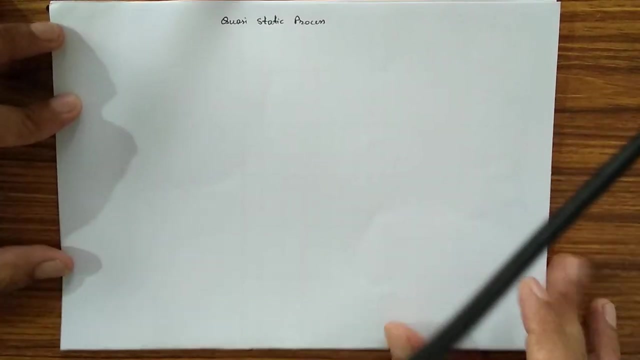 equilibrium, So a process which is carried out very slowly, with small gradient, and in each state the system remains in thermodynamic equilibrium. So in this case, quasi-static process is the central function of the system. This is also called a quasi-static process. So what is quasi-static process Now? Firstly, we will 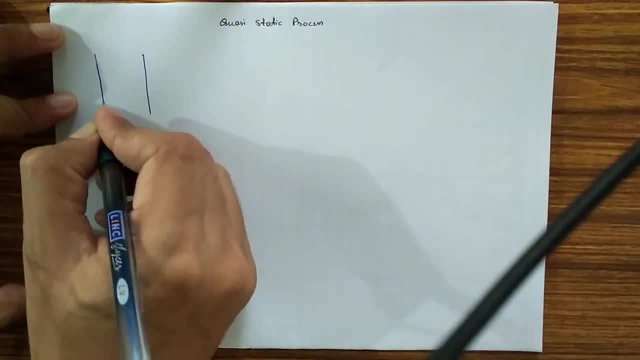 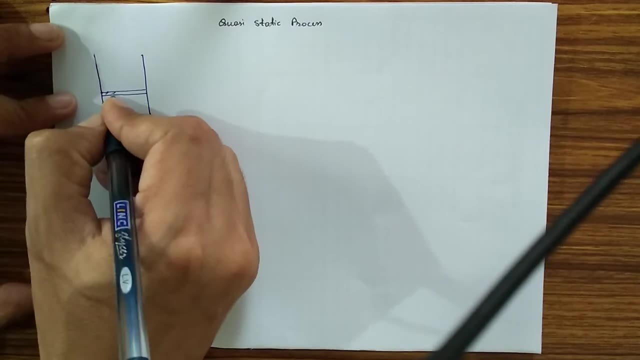 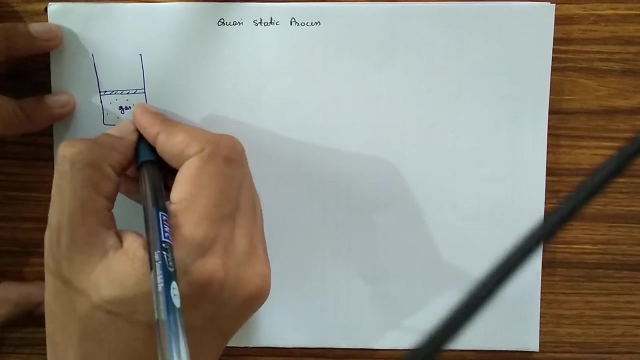 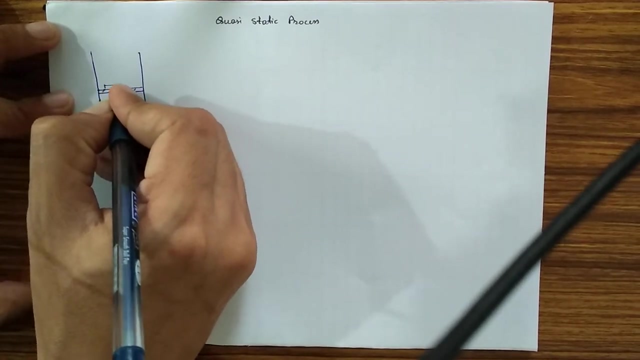 start with an example of a system as well: A gas случie huh. So let's see the system. Let us consider a gas cylinder. This is a piston cylinder system, This is a piston and these all are gas. so, and which is here that we have kept differential weights? 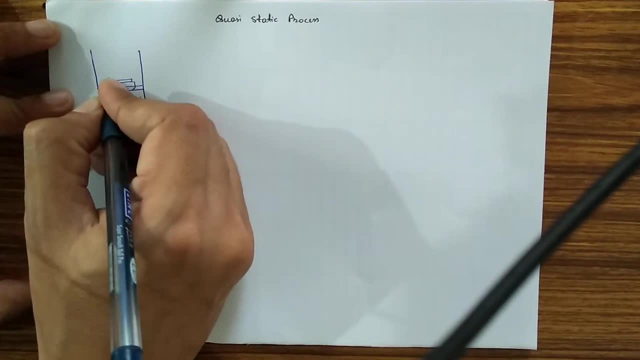 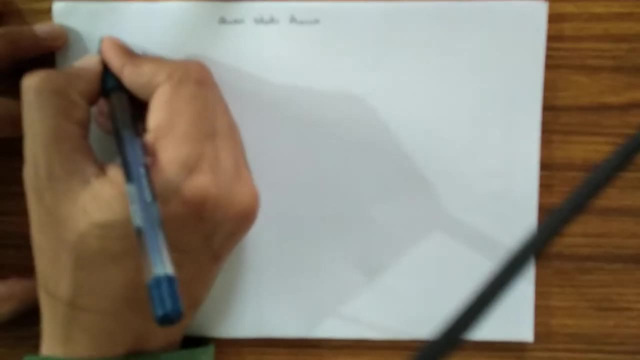 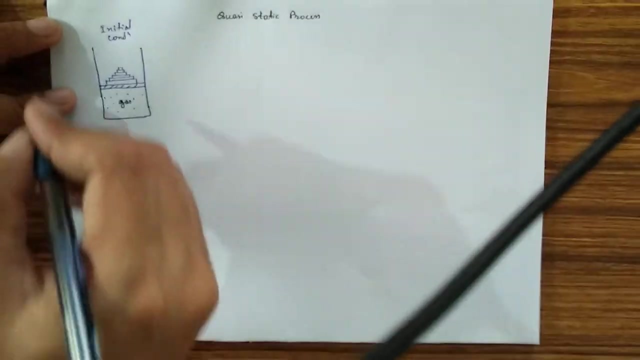 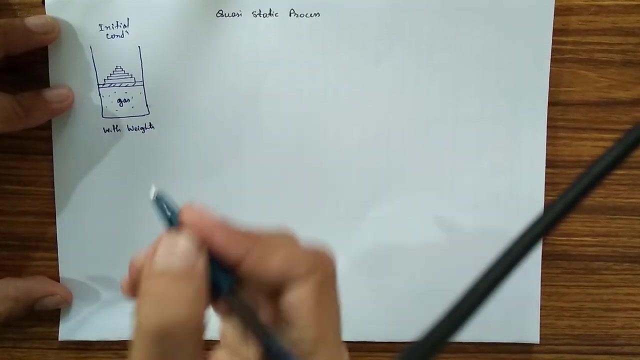 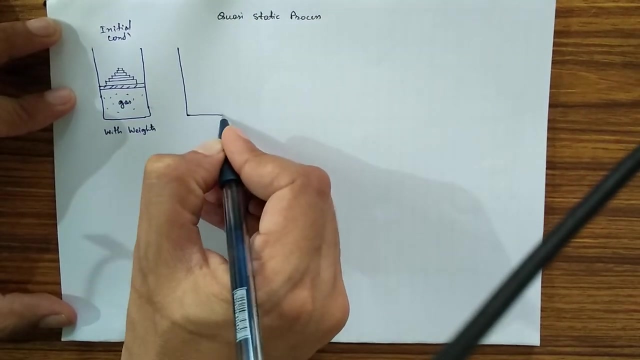 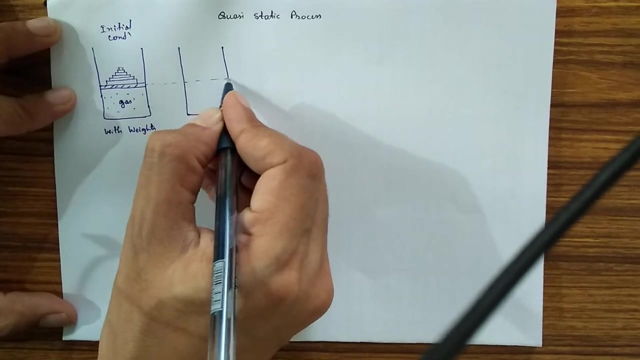 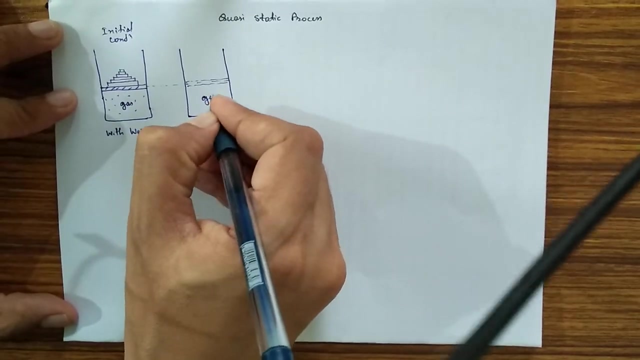 very small weights. let's see this one. these are differential weights. so this is the initial condition of the system with weights, with the differential weights. so if we see, if we remove these weights one by one, let's see what happens here. this is the initial condition, the system, the same we are drawing here, the same system. so let's first remove this one small weights. 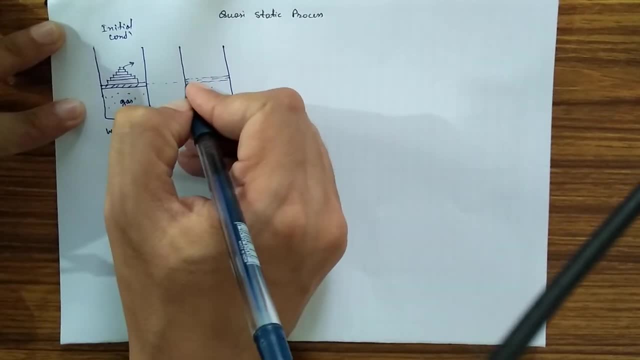 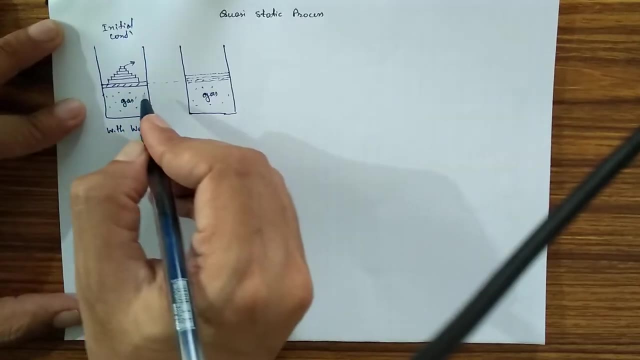 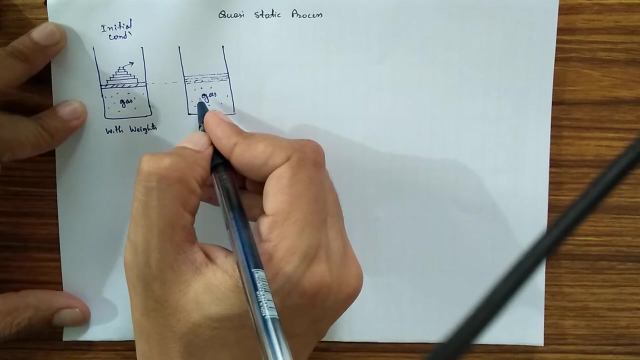 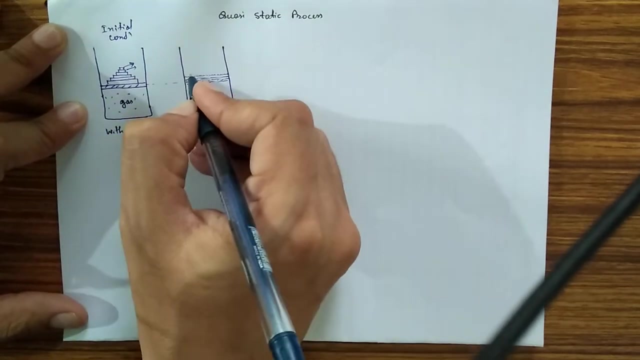 as we remove these weights, then this piston, this piston will go further up. this is the system. this is done very slowly. so after moving this system, this, the stains, the system comes to equilibrium, that is, there is thermodynamics. equilibrium is achieved. after that we remove another weight again, the piston will move up and in this state also the 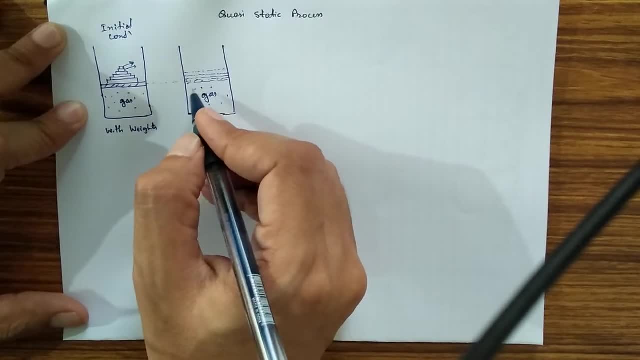 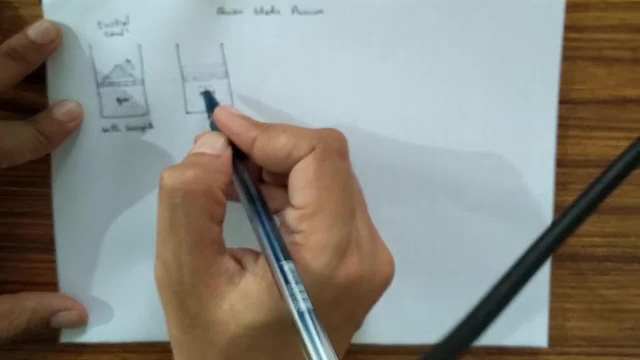 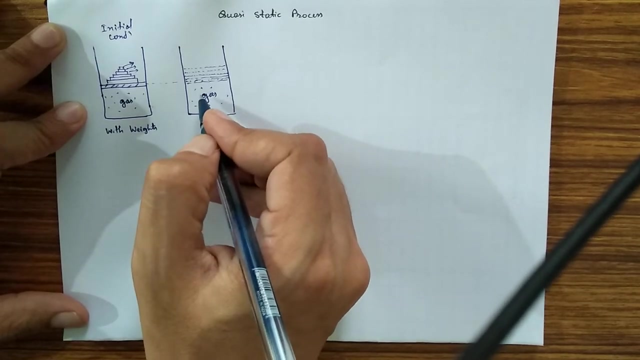 thermal will comes to. sorry, the system will comes to thermodynamic equilibrium again. we will remove this weight, the piston will move a little bit up and since the process is very slow, so it will get time to achieve equilibrium- equilibrium- the system will comes to thermodynamic equilibrium. similarly, we 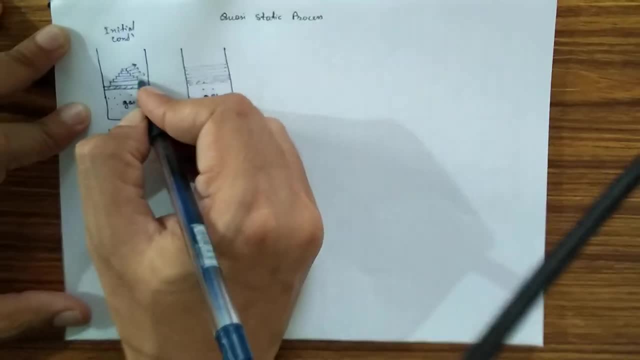 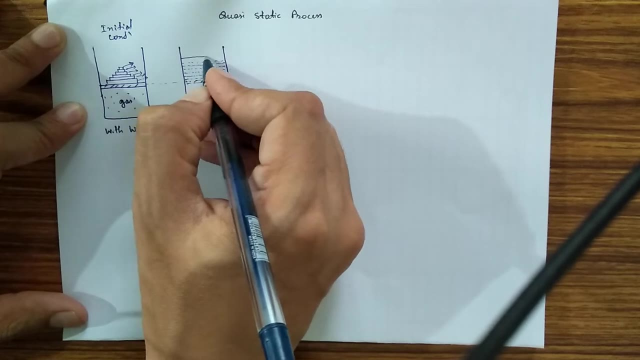 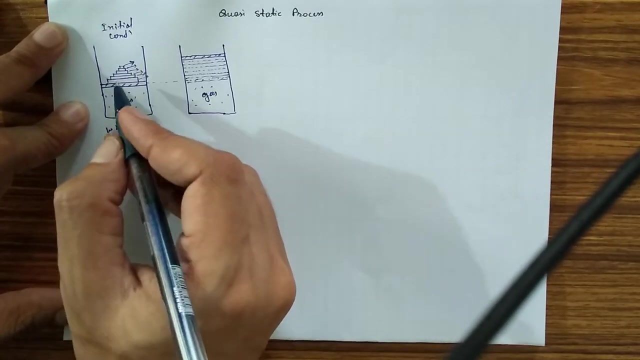 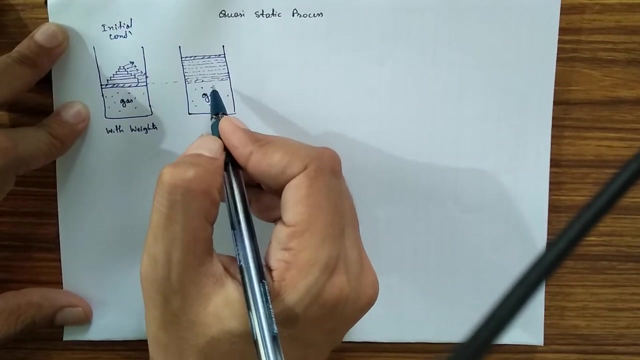 will remove this, the piston will move here. we will remove this, the piston will move here. and finally, this will remove this one, the piston will comes here. so what we see, since we are removing this weights one by one and in very slow manner, so that after removing one weight, the system comes to thermodynamic. 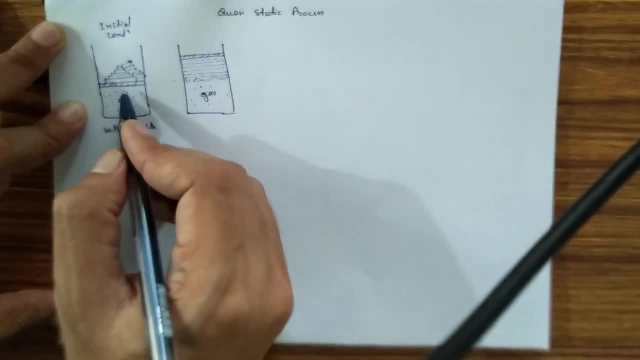 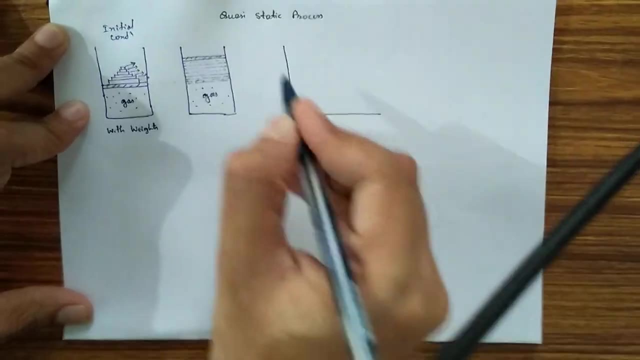 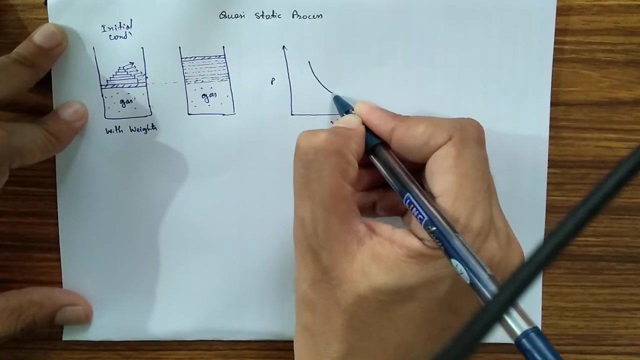 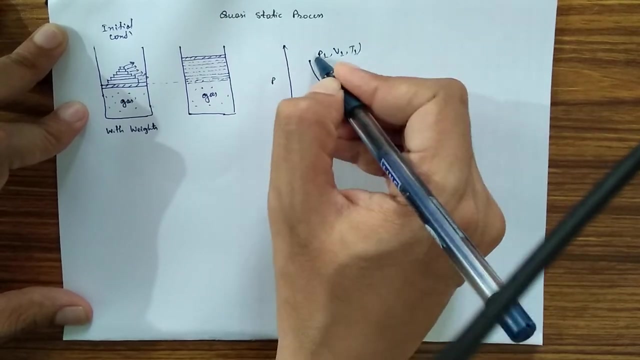 equilibrium, then the other weight is removed. so this process is carried out very slowly. we can see this in PV diagram. this is our pressure volume curve. you will see, we will achieve this curve. initially we have pressure P 1, volume V 1, temperature T 1.. 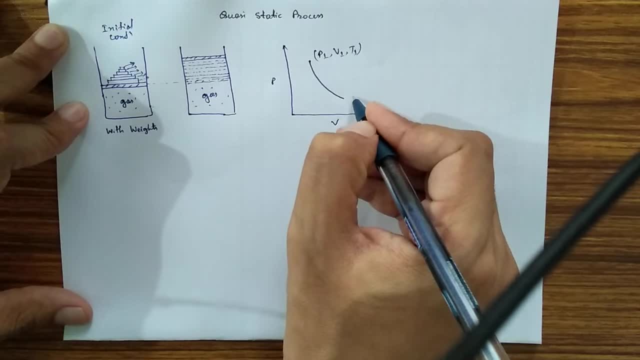 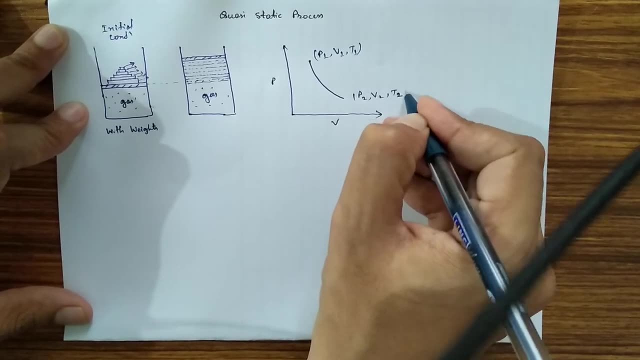 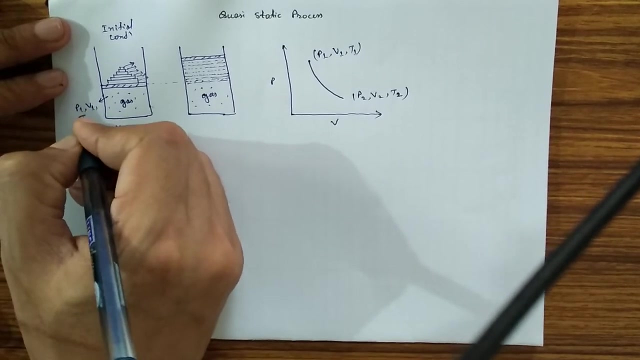 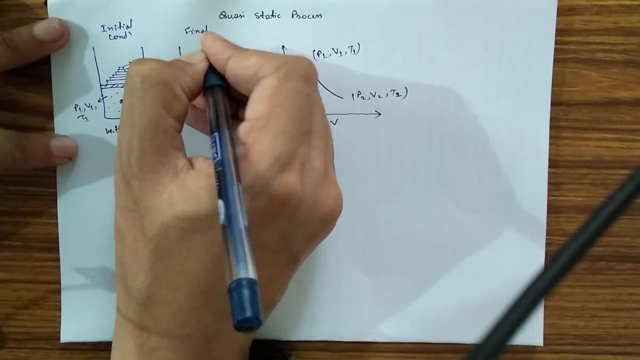 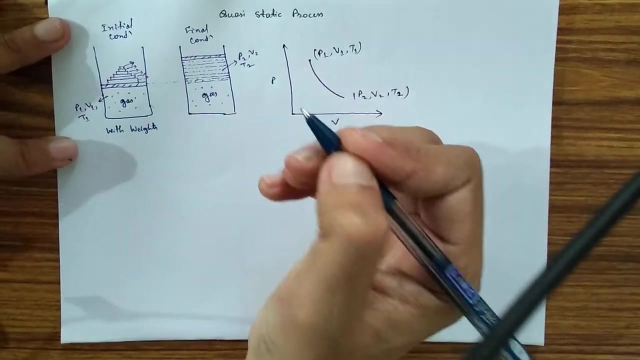 This is condition and finally, we have achieved pressure P2, volume V2 and temperature T2. this was the initial condition where P1, V1, T1 and this is the final condition. final condition: here the pressure is P2, V2 and temperature is T2. 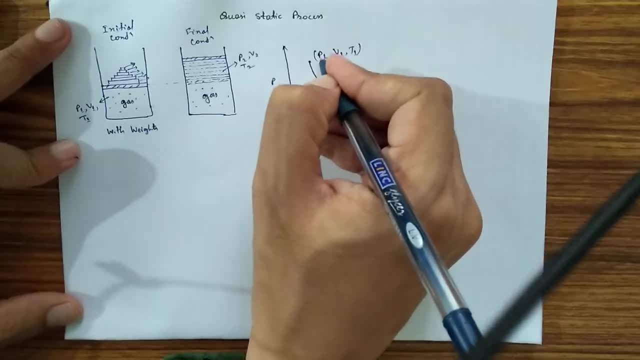 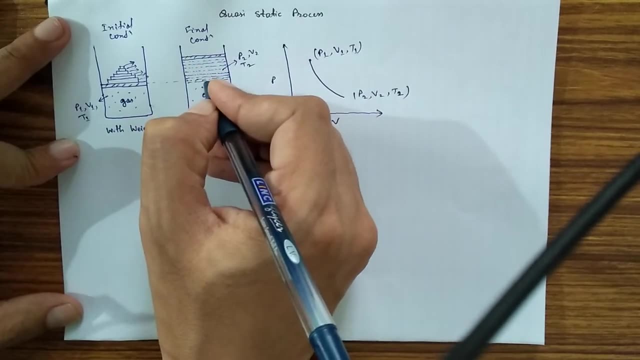 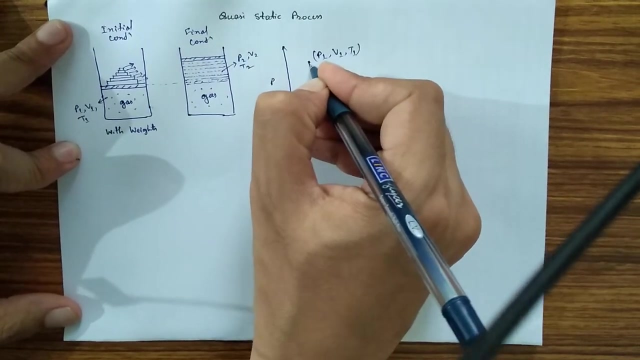 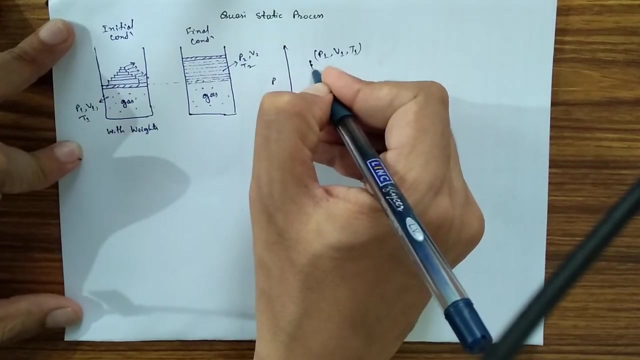 so if we see that initially we have pressure, volume and temperature after removing this first weight, the system goes. that does this. this though: this is the piston that moves up, so we will have this curve here at this point, and after achieving equilibrium, we have removed the next weight. again, the system goes to. 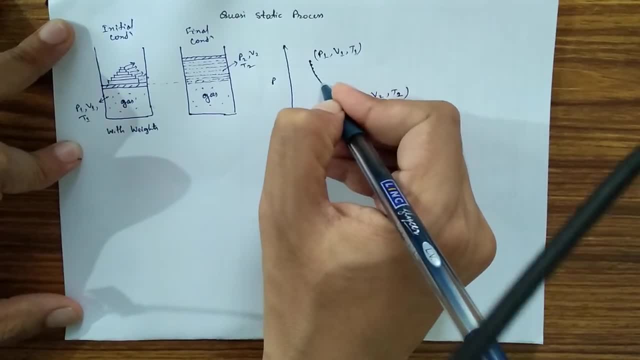 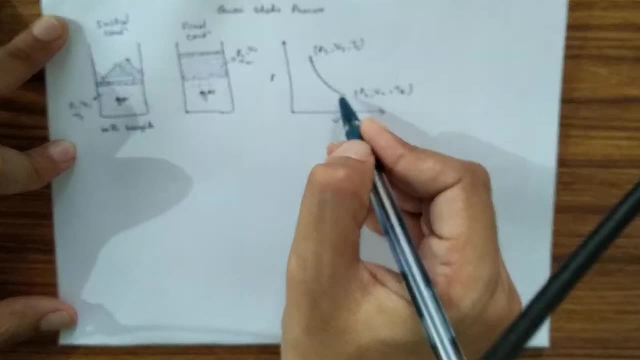 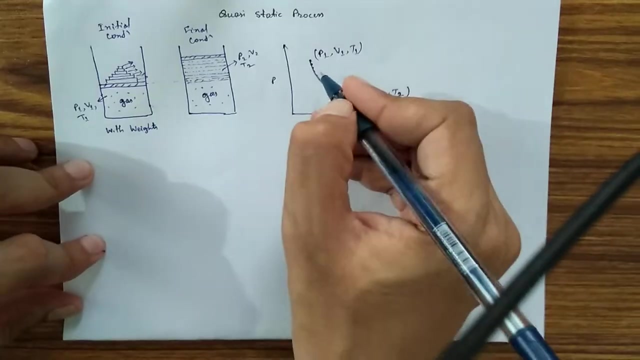 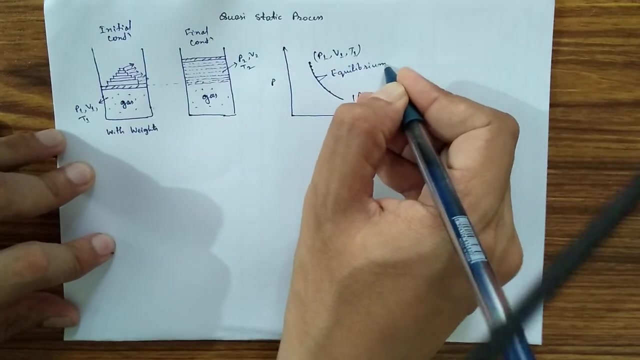 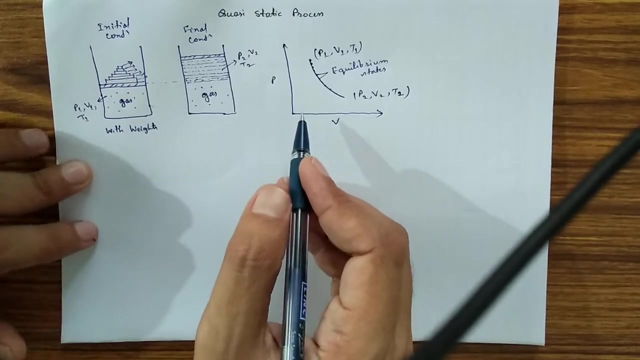 thermodynamic equilibrium. similarly, in each step the system is under thermodynamic equilibrium and since we have removing the weights, the pressure is decreasing and volume is increasing. we can see from the graph also. so, in each step, in each state, these are the states, equilibrium states. so in each the system is in thermodynamic equilibrium. so we can. 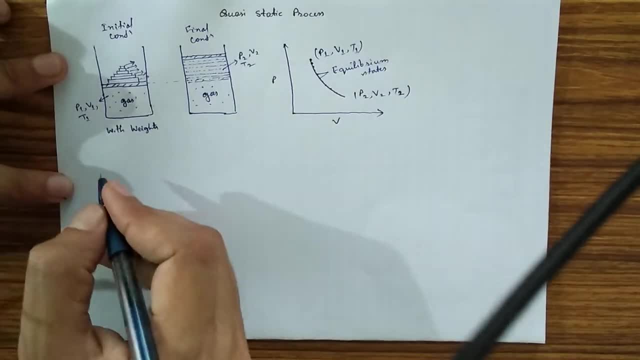 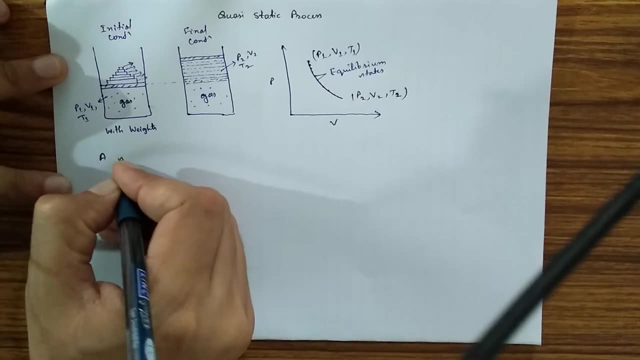 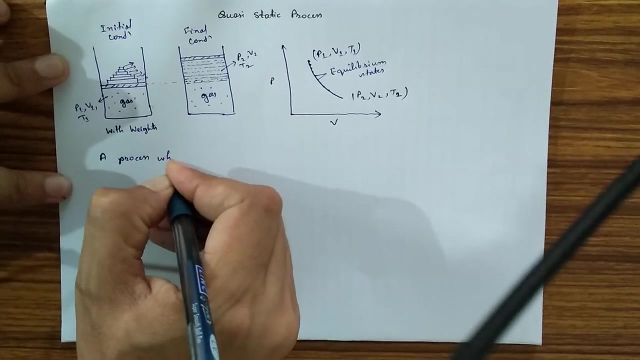 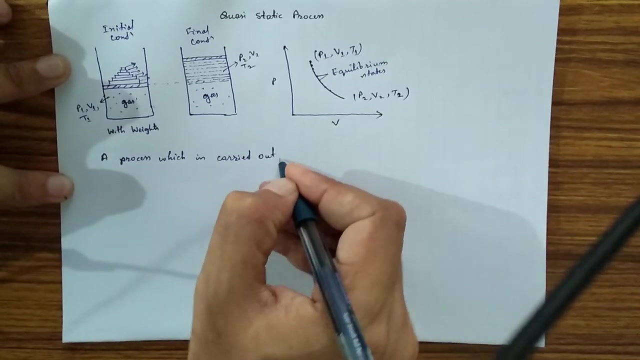 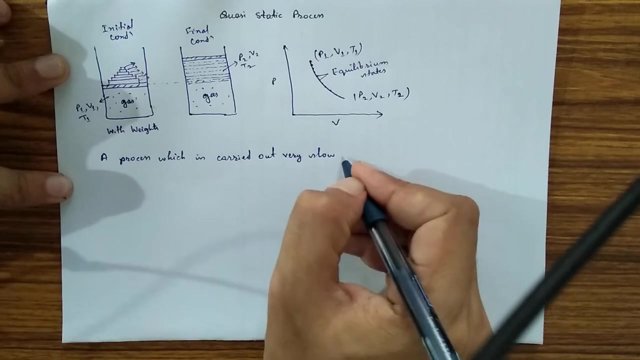 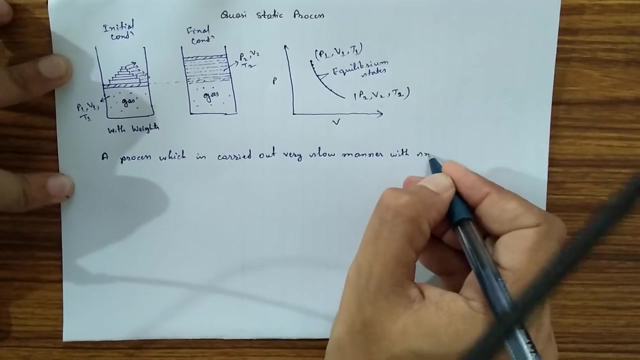 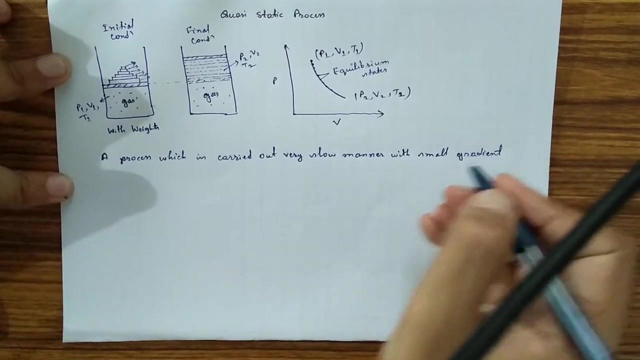 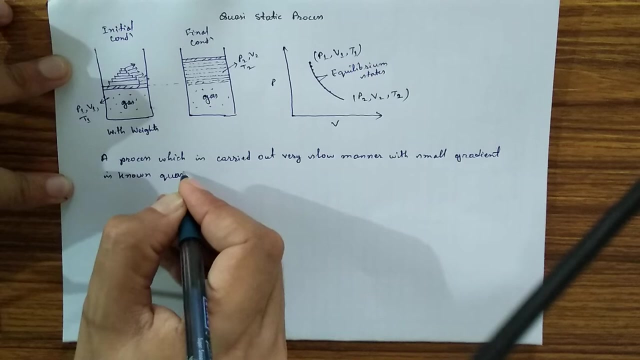 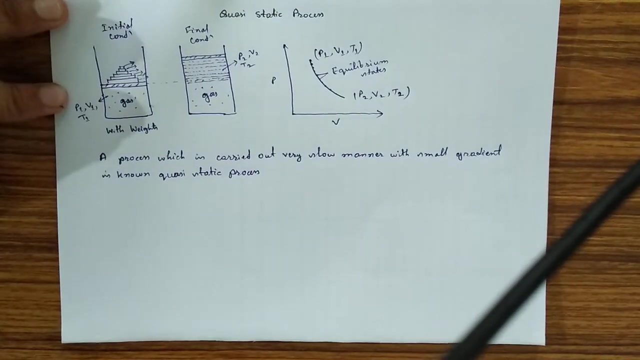 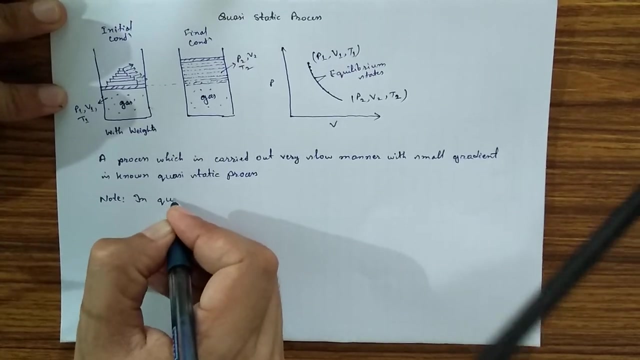 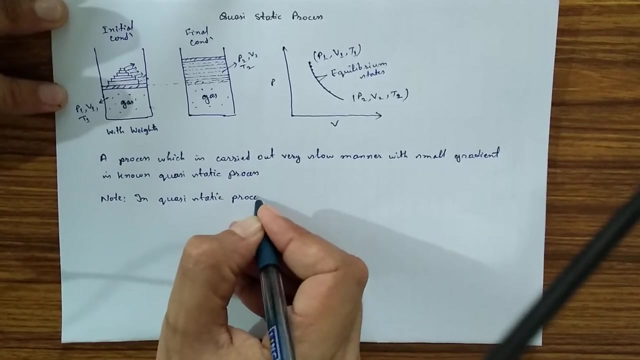 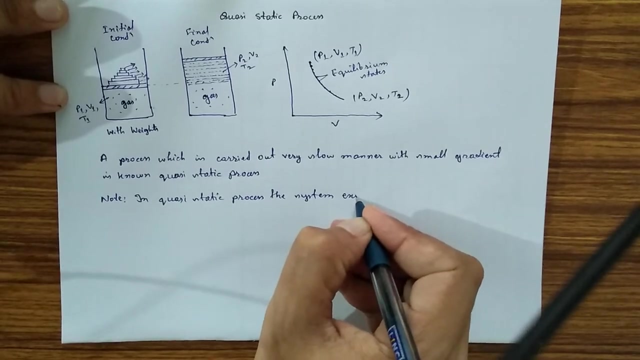 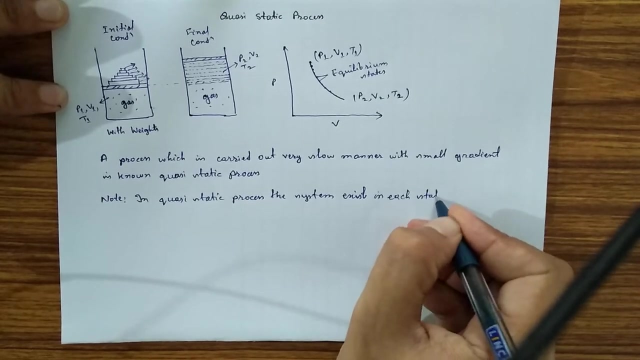 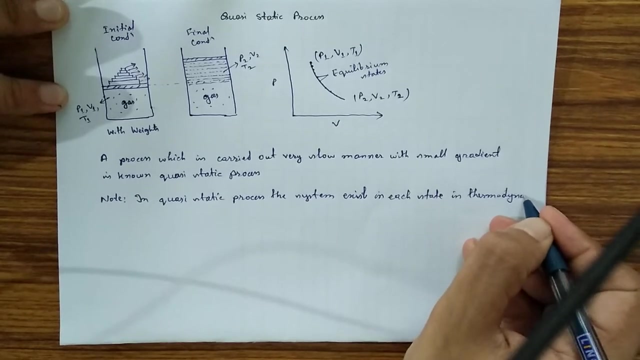 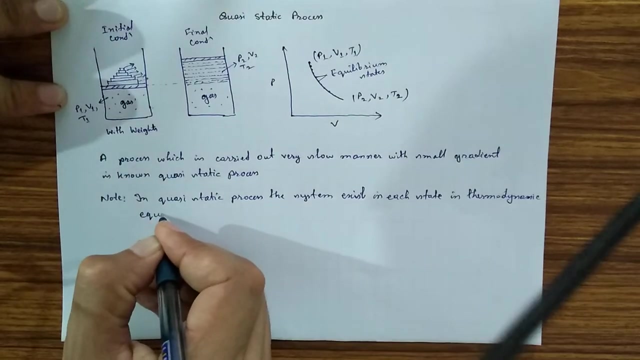 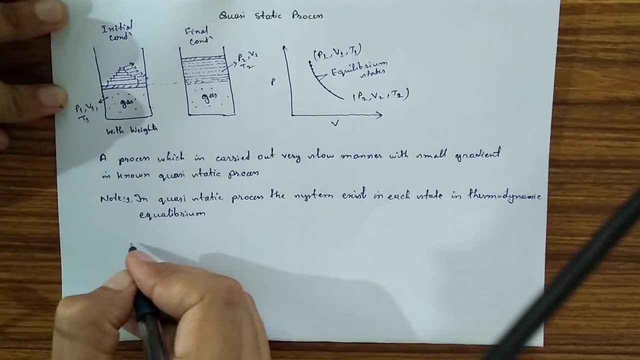 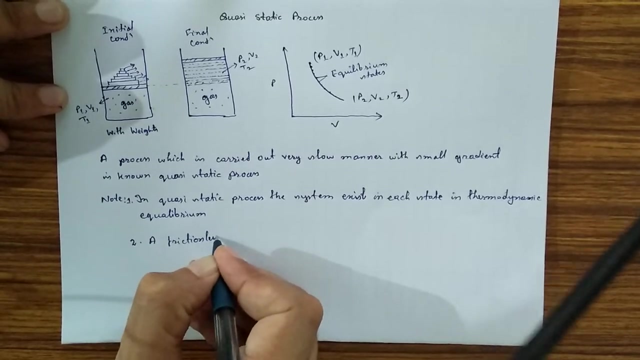 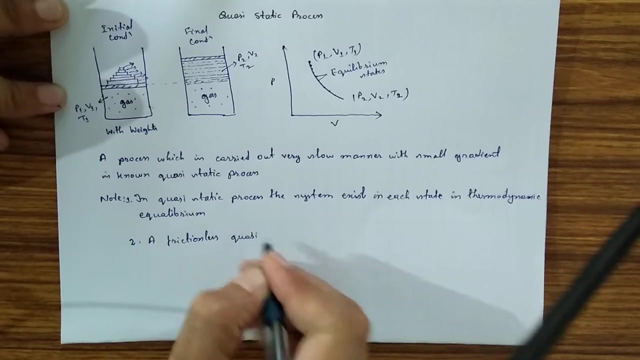 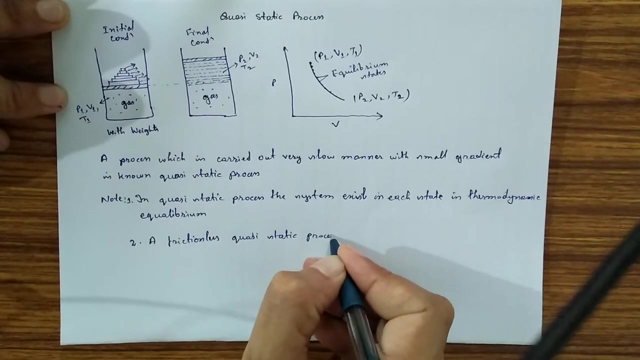 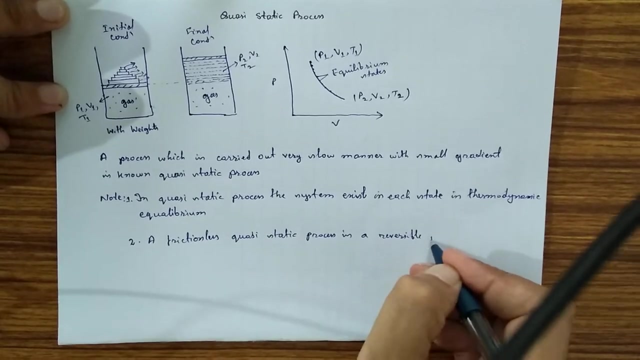 somewhere in this Och Pedersen, which is carried out out very slow manner with small gradient, is known as quasi static process. we can note that in quasi static process the system exists in each state in thermodynamic equilibrium. this was the the note 1 and note 2: a frictionless. a frictionless, quasi static process is a reversible process. 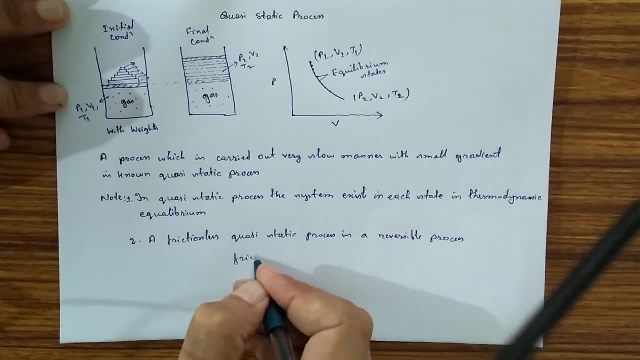 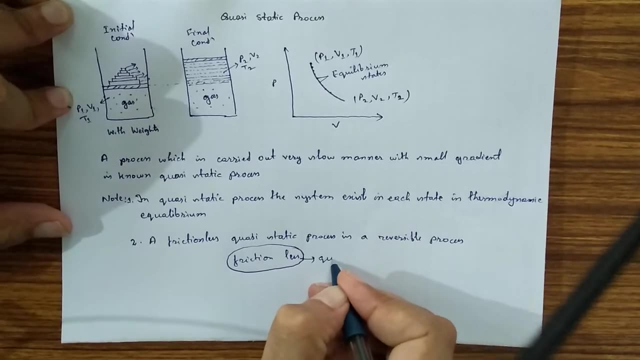 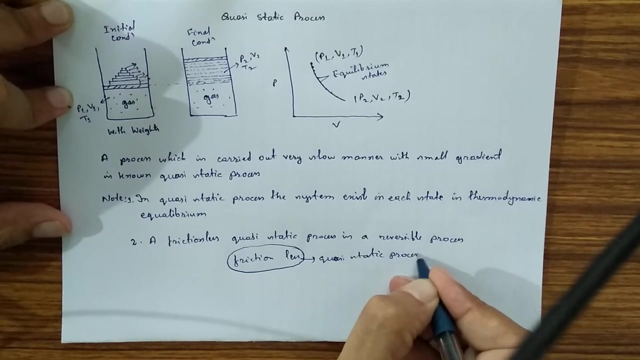 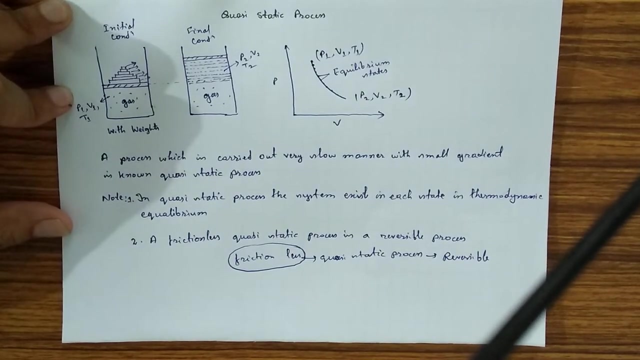 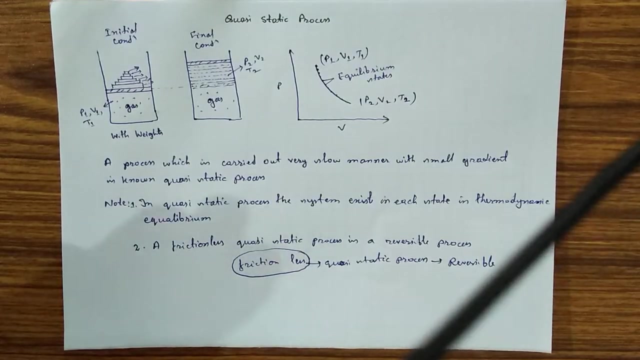 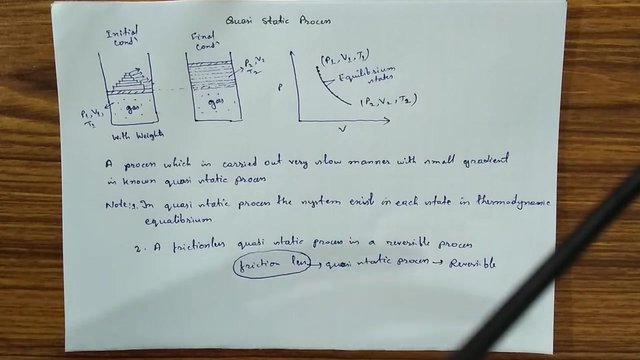 so a frictionless, quasi static process process is a reversible process. so a frictionless, quasi static process is a reversible process. so so, so we have seen that what is quasi static process? it is a process which is carried out very slowly, such that in each state the system remains in thermodynamic equilibrium. 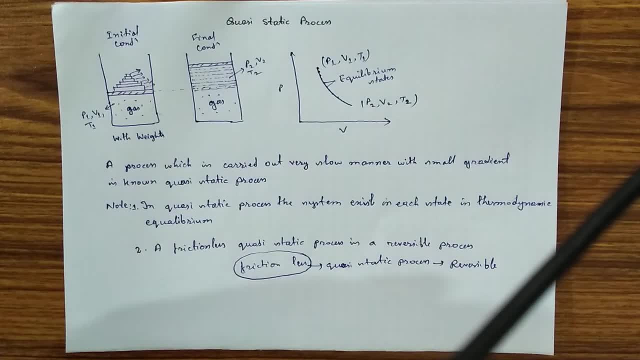 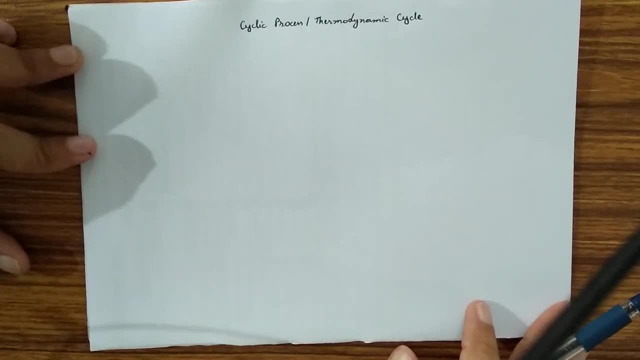 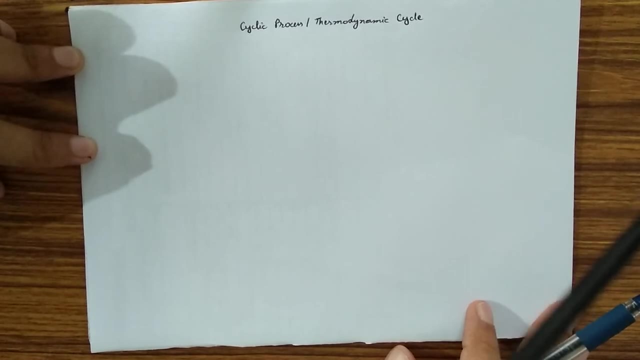 and a frictionless, quasi static process is a reversible process. now we will see cyclic process, that is, thermodynamic cycle. so a system is said to have undergone a cyclical process cycle when initial and final points are same. so a cycle is said to be. so. that is a system has. 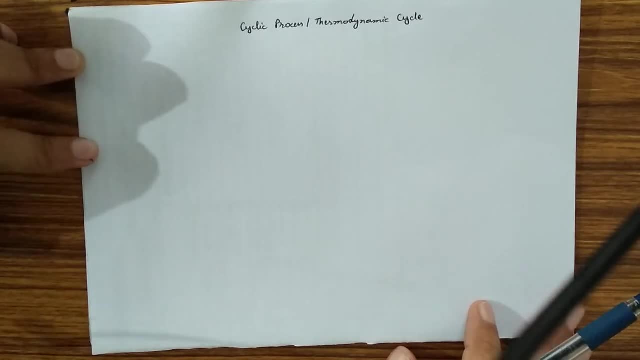 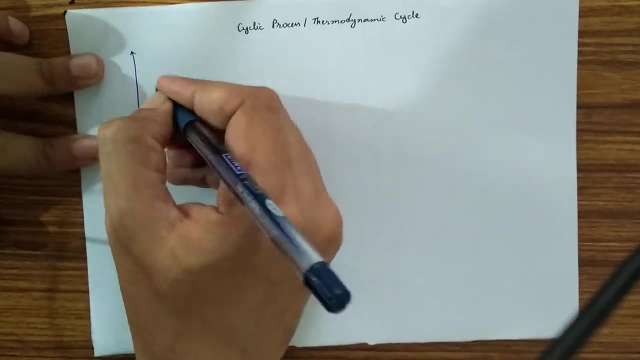 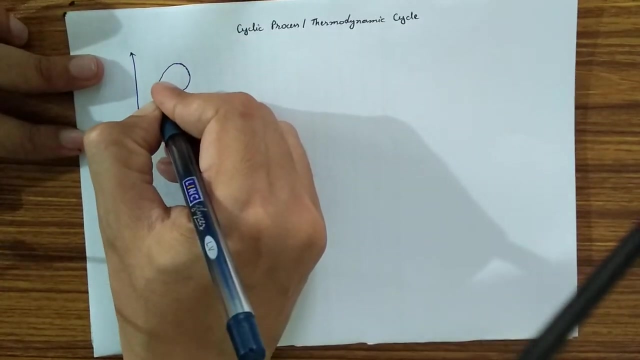 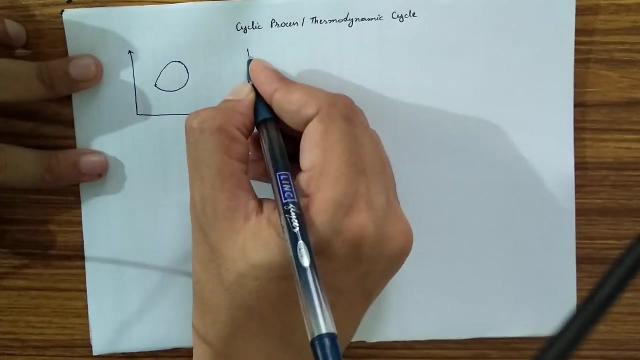 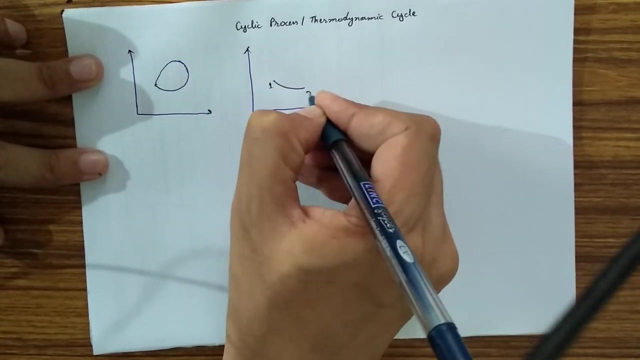 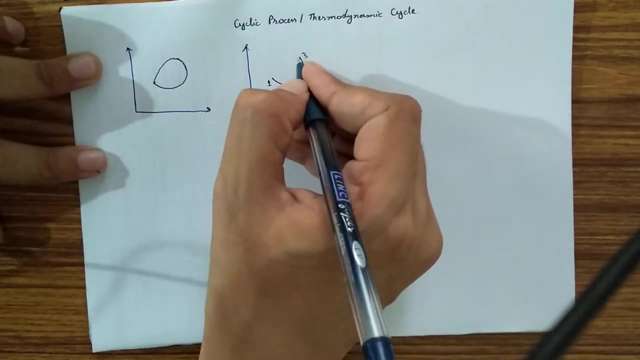 undergone a cycle when initial and final points are same. let's see this: we have started a process from here and it is, it is ending here. so the initial state was this and the final was also the same. this is- let us consider another example- a process from this: 1 to 2: this is a process. 2 to 3 is another process, and 3 to 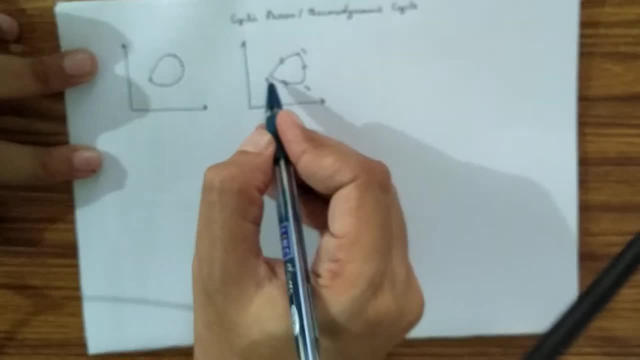 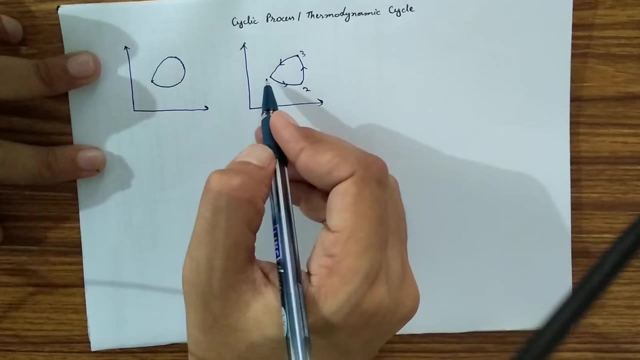 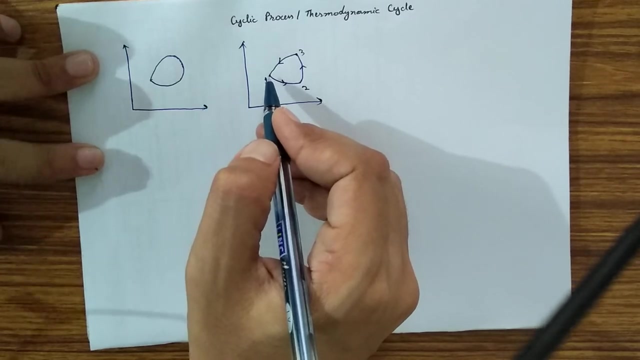 the process. since we have started from process, from state 1 to 2, one process. state 2 to 3 are the process and 3 to 1, another process. the initial state will end again from here. a sta y other process. stay stage was this and the final stage is the same. so this has undergone a cycle. this is 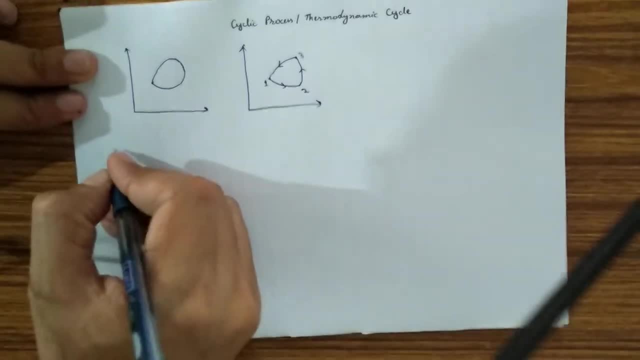 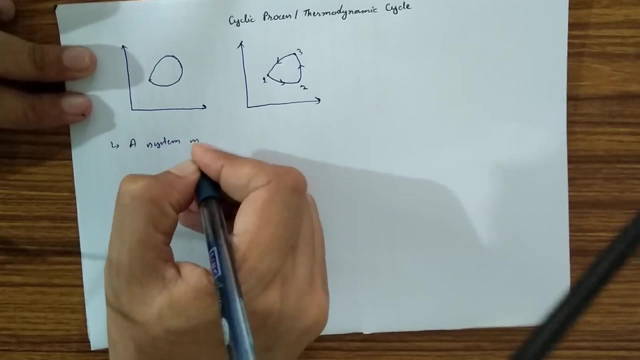 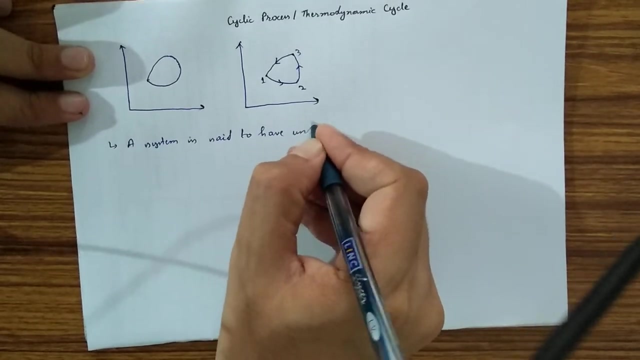 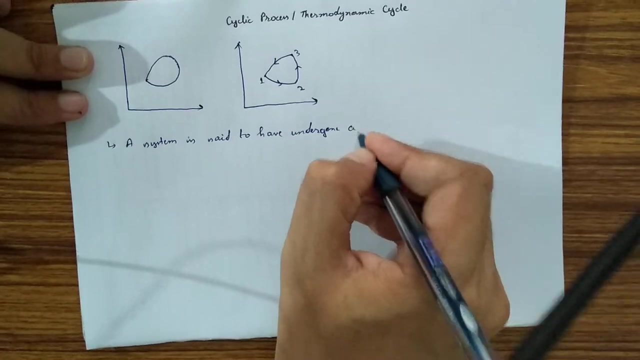 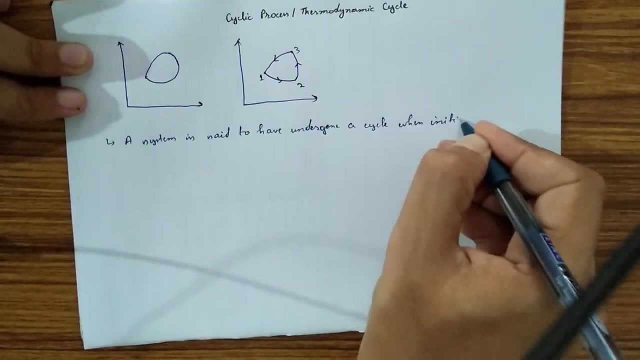 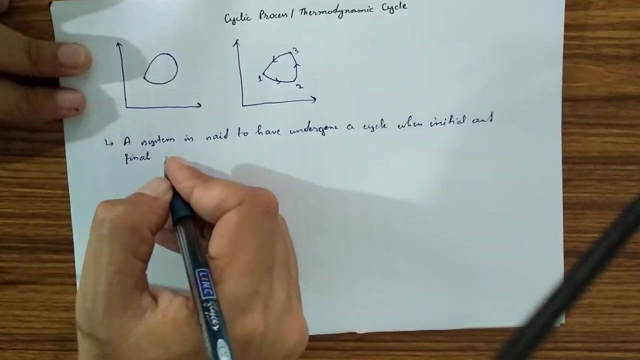 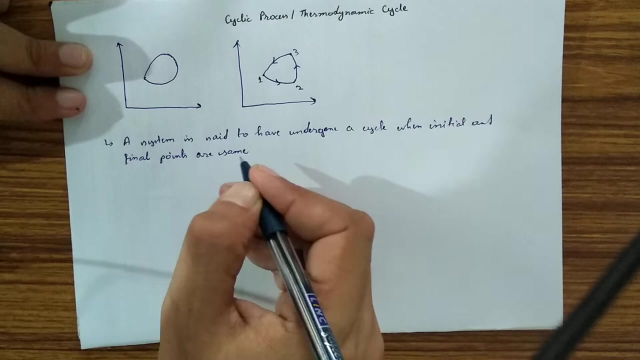 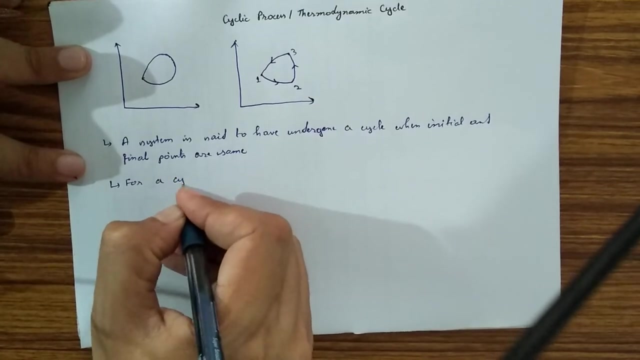 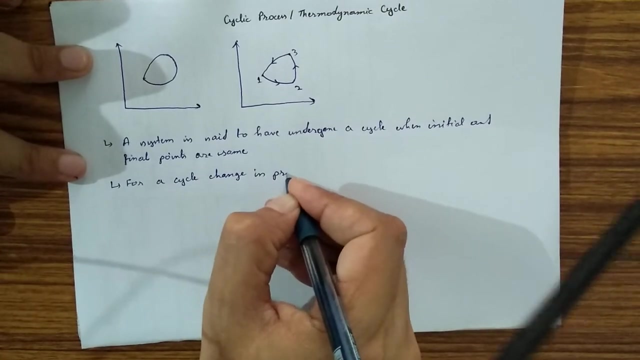 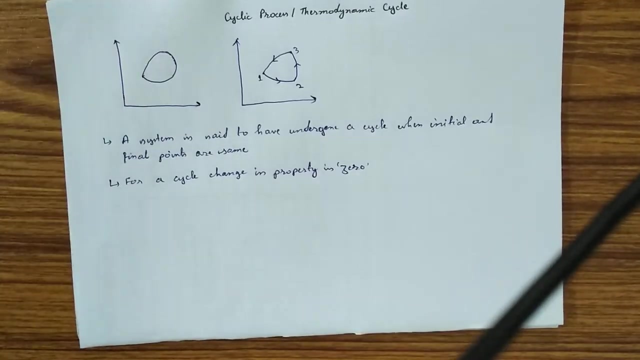 called as cyclic process or thermodynamic cycle, a system is said to have undergone undergone a cycle when initial and final points are same and, for a cycle, change in property is zero. so a system is said to have undergone a cycle when initial and final points are same and, for a cycle, change in property is zero. 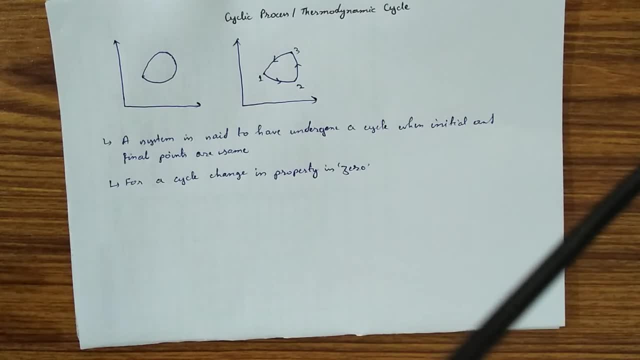 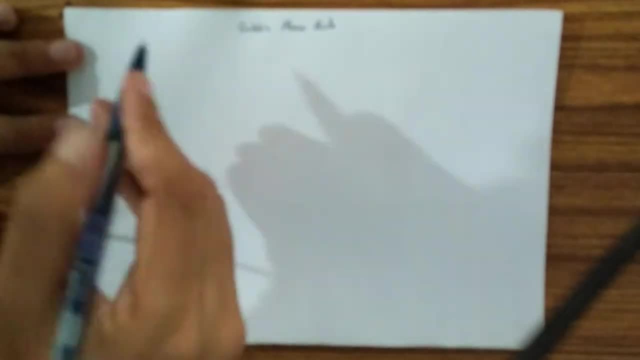 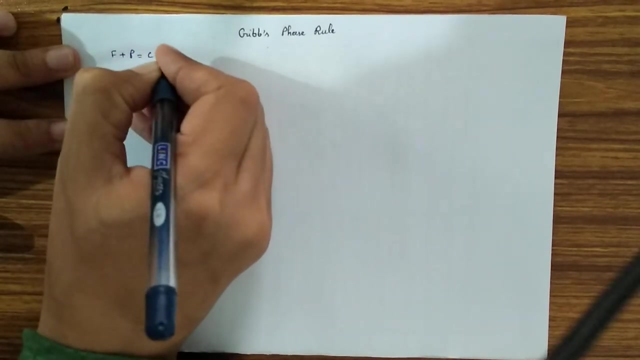 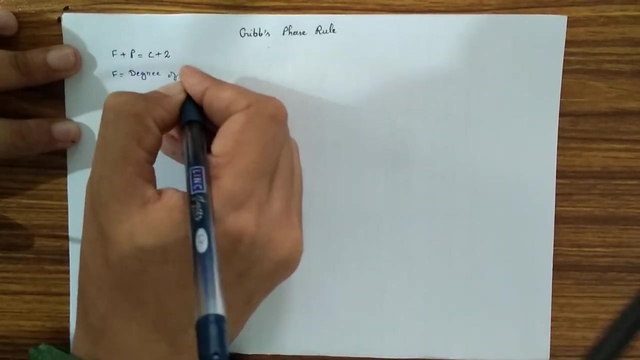 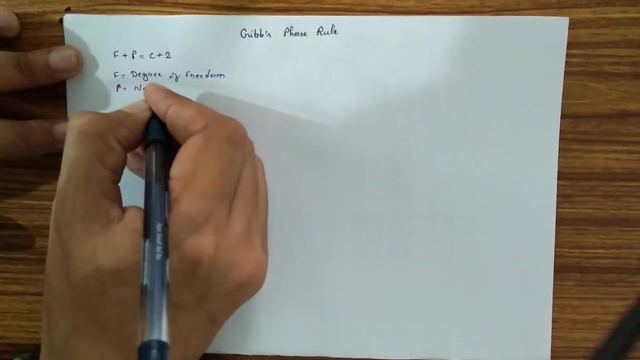 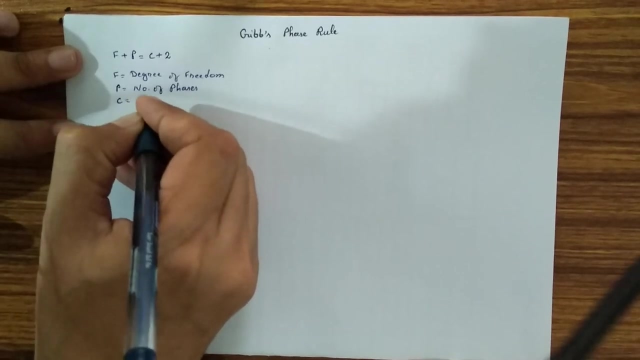 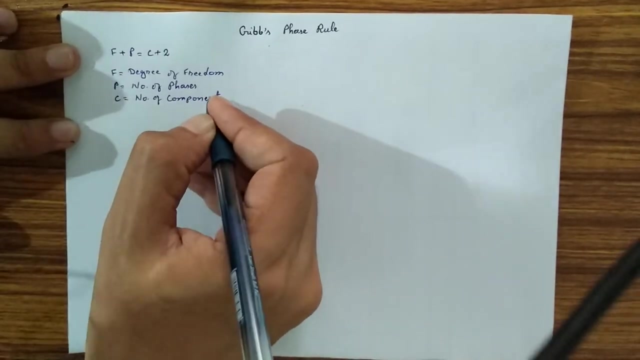 so this is called as cyclic process or thermodynamic cycle gives phase rule. so let's see what is give phase rule: f plus p is equal to c plus 2. where f equals to degree of freedom, p is equal to number of phases, c is equal to number of components. 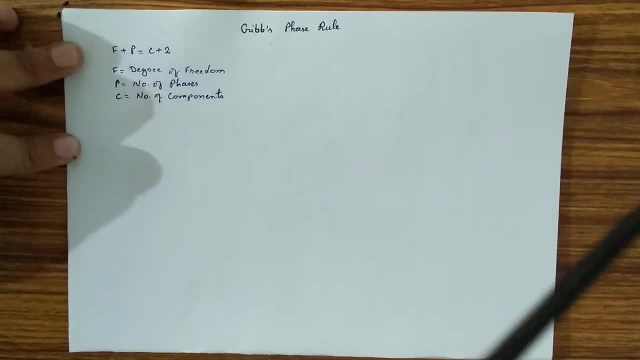 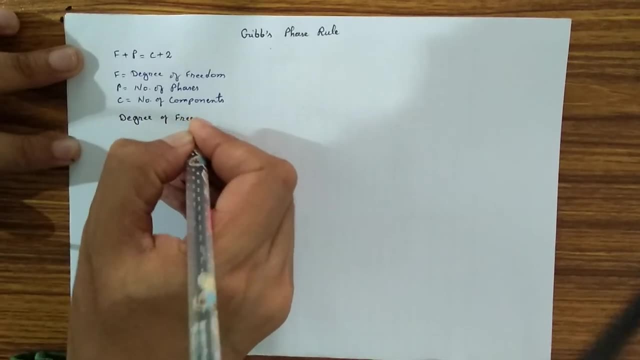 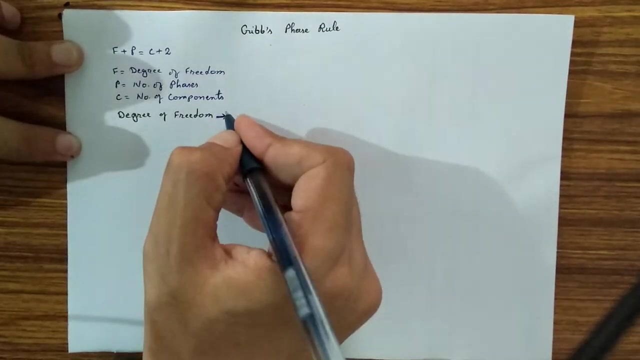 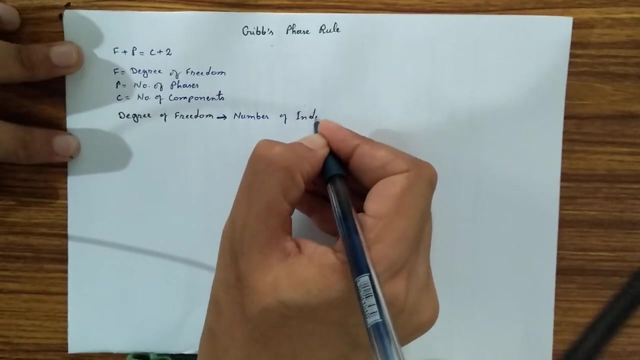 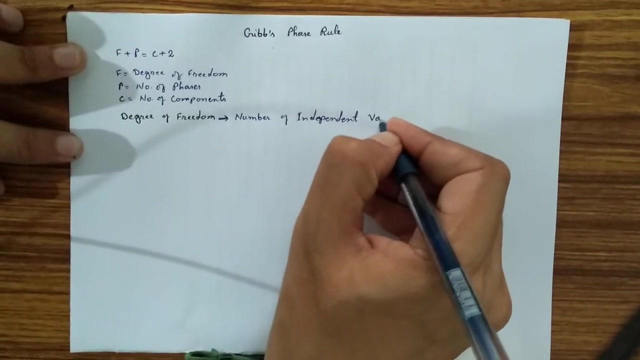 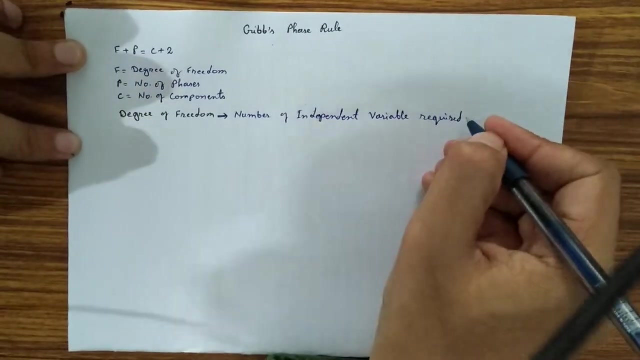 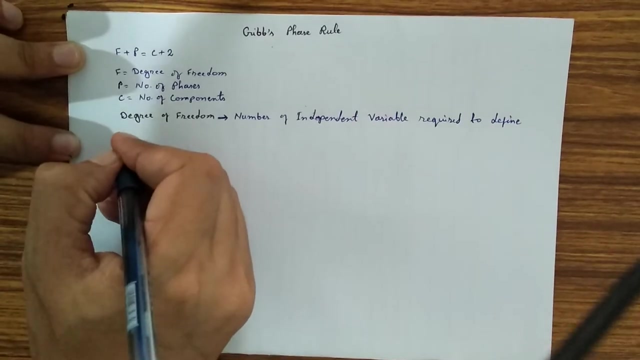 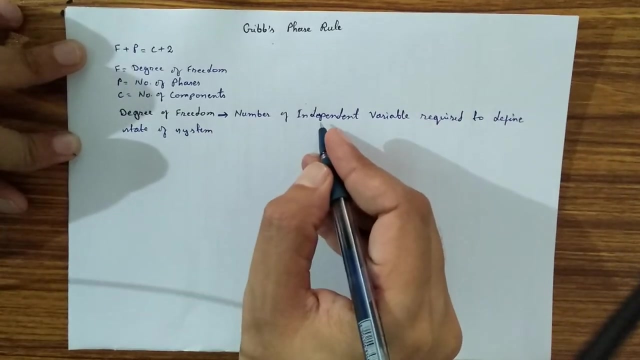 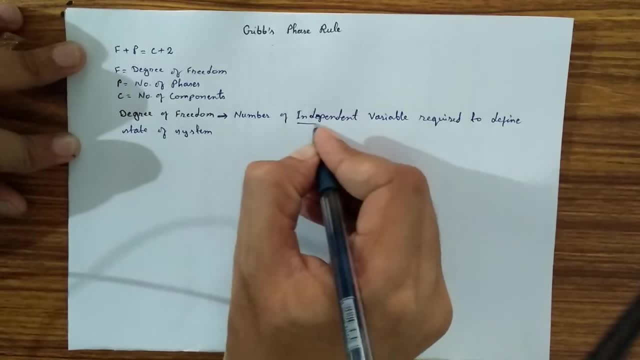 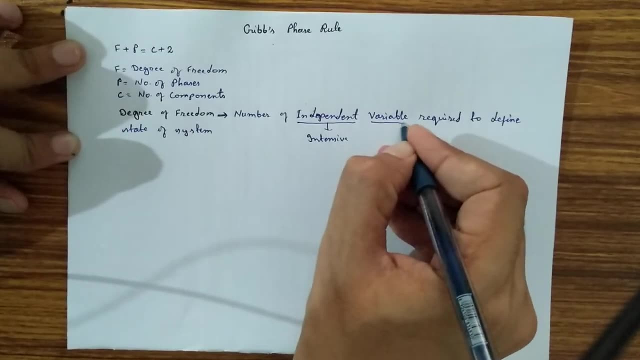 it is the number of independent variable. it is the number of independent variable required to define, required to define state of system. here independent means state of system. here independent means state of system. here independent means intensive, variable means property, so degree of freedom. it is the number of. 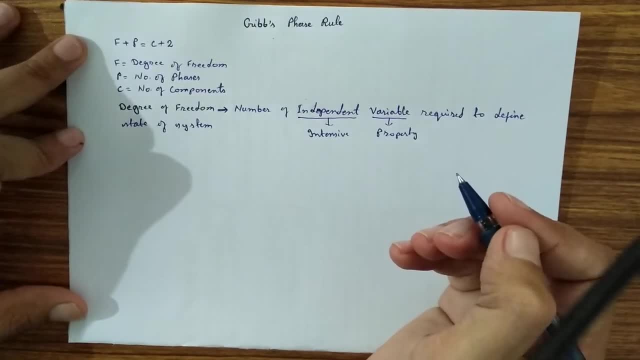 so degree of freedom, it is the number of so degree of freedom, it is the number of independent variable required to define independent variable required to define independent variable required to define state of a system. or we can say it is state of a system, or we can say it is. 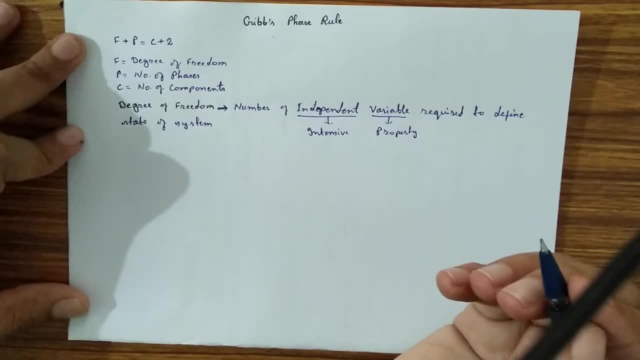 state of a system, or we can say it is the number of intensive property. the number of intensive property, the number of intensive property required to define state of the system, required to define state of the system, required to define state of the system. state of the system means condition of. state of the system means condition of. state of the system. means condition of the system. the system to define the condition of the. the system to define the condition of the system, that is, the state of the system. the system to define the condition of the system, that is the state of the system. 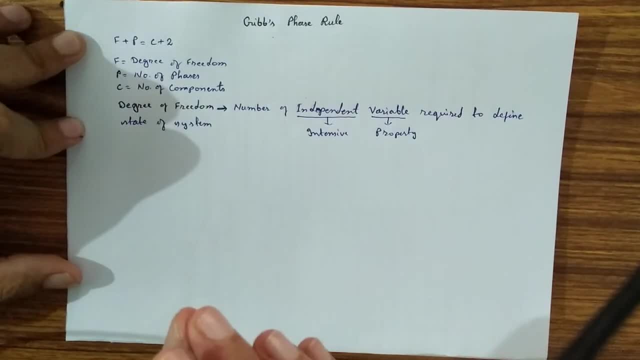 the system to define the condition of the system. that is the state of the system. what is the number of? that is the state of the system. what is the number of? that is the state of the system. what is the number of independent variable required? this is independent variable required. this is: independent variable required. this is that is called degree of freedom. that is called degree of freedom. that is called degree of freedom. so degree of freedom can also be written. so degree of freedom can also be written. so degree of freedom can also be written as number of- sorry, intensive. 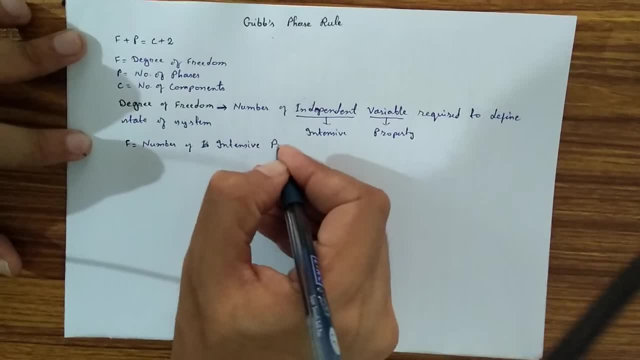 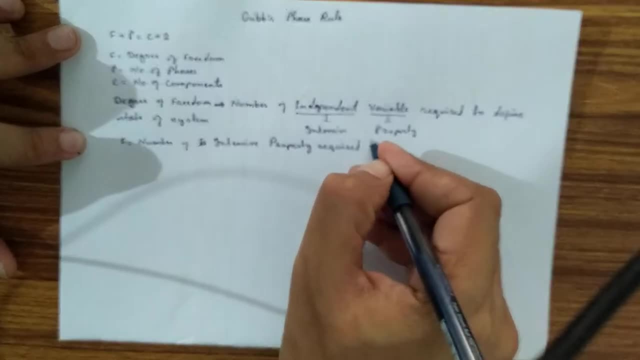 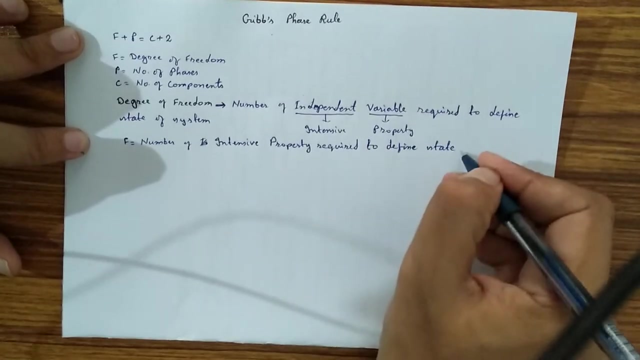 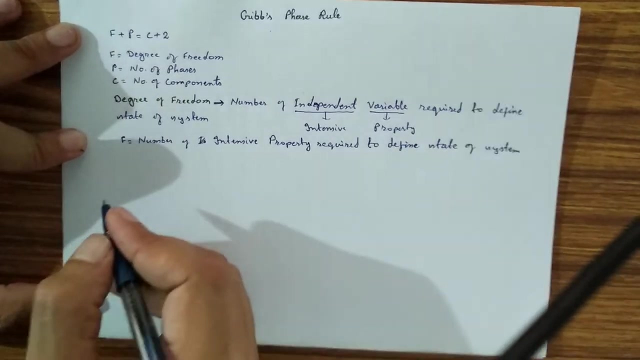 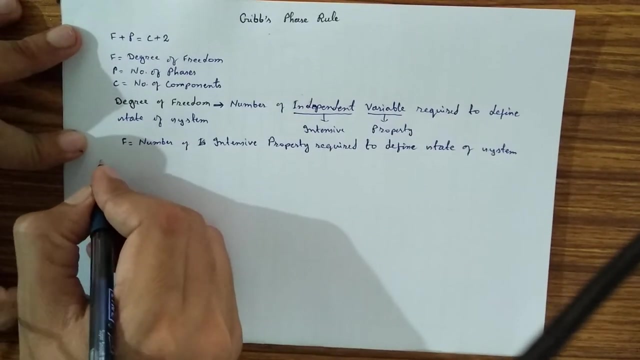 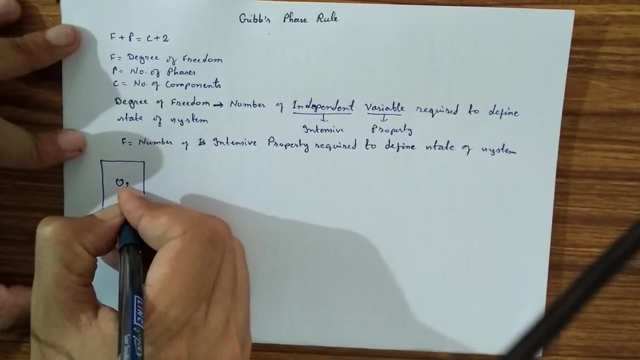 intensive, intensive property, property, property required to define, to define, to define state state, state of system, of system, of system. this will be understood easily if we will take an example. let us consider one container which is having O2 inside. so this container is having oxygen gas, that is, it is having 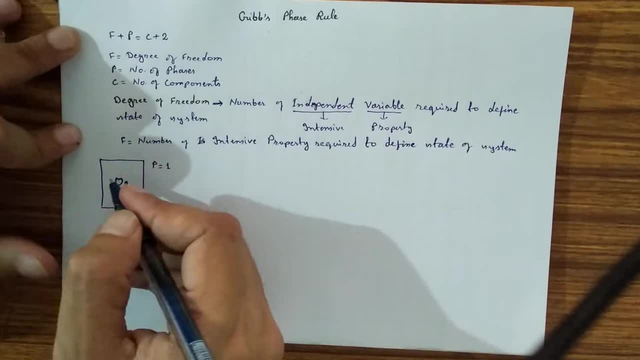 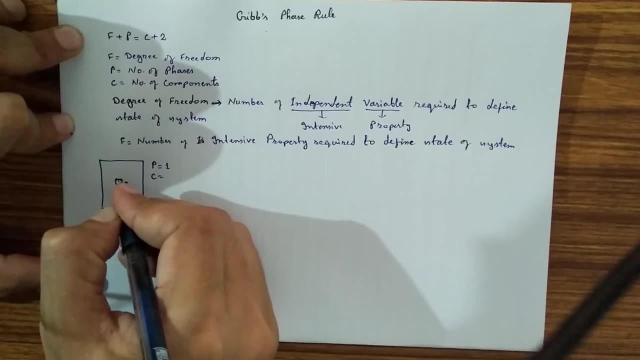 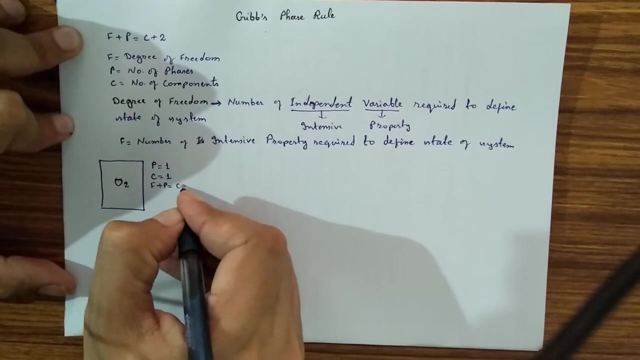 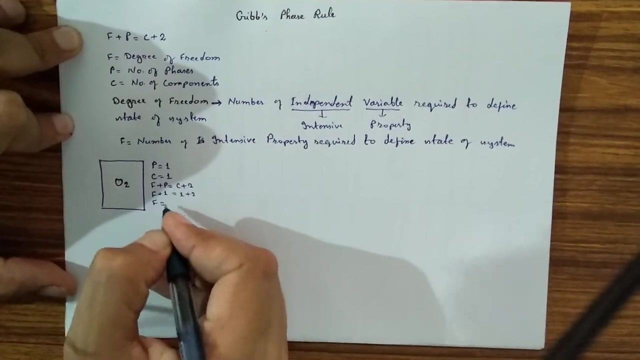 phase 1, since oxygen is present in only one phase here, in gases form. so number of phase is 1. only one oxygen is there, so number of component is also 1. using the formula F plus P equals to C plus 2, F plus 1, 1 plus 2, we will get degree of freedom as 2. so here the 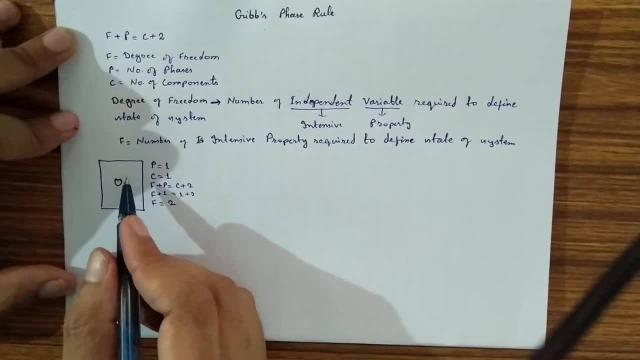 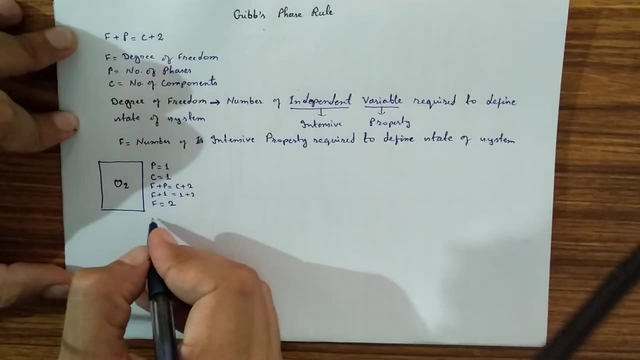 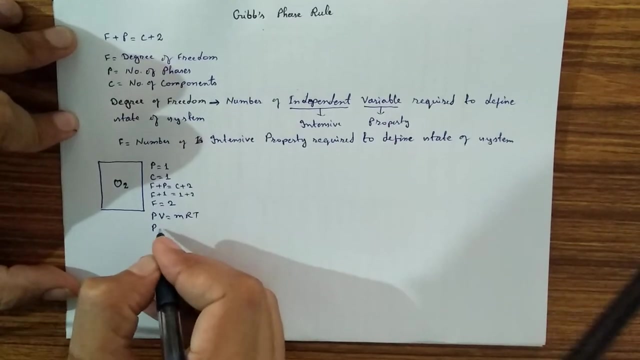 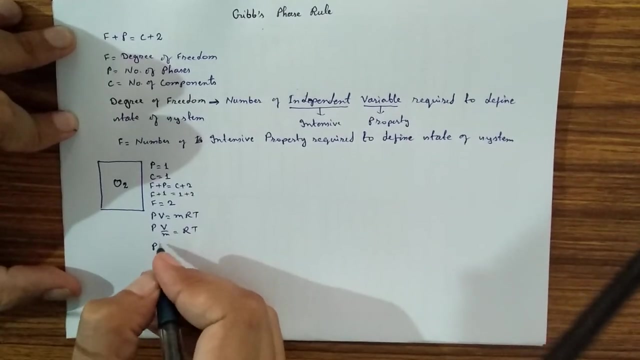 minimum independent variable required for this is 1.. to define the state of the system is 2, because degree of freedom is here 2. we can understand it easily by see: this is PV, equals to MRT, so P if we put bring M here V by M, RT volume. 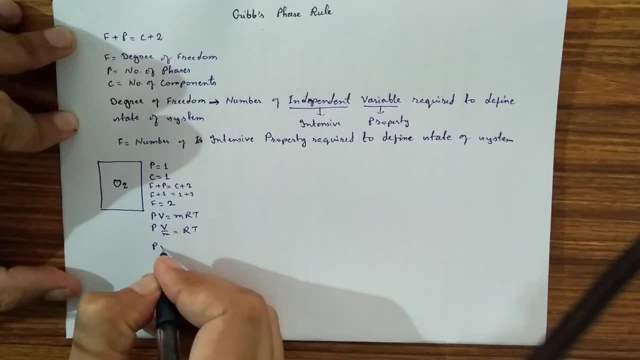 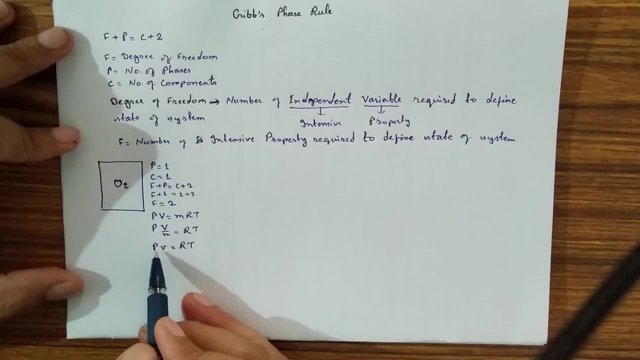 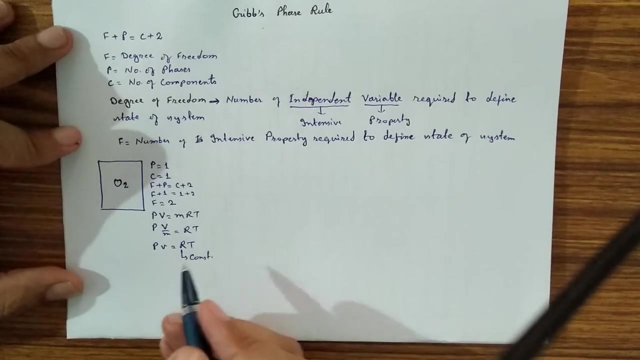 per unit mass. this is a specific volume we can. this is divided by small, v equals to RT. so if we know two variables, like if we know temperature or pressure, because R is a constant, this is a gas constant, this is constant here. so if we know the temperature or pressure, we will. 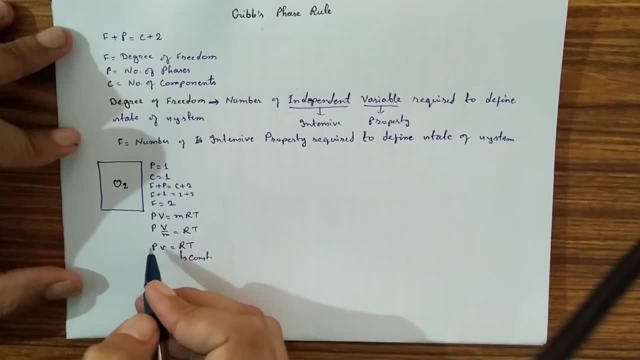 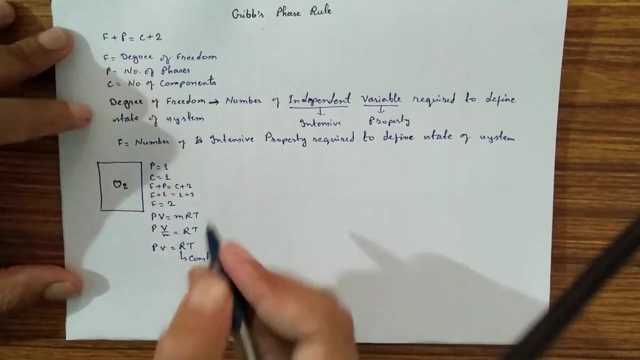 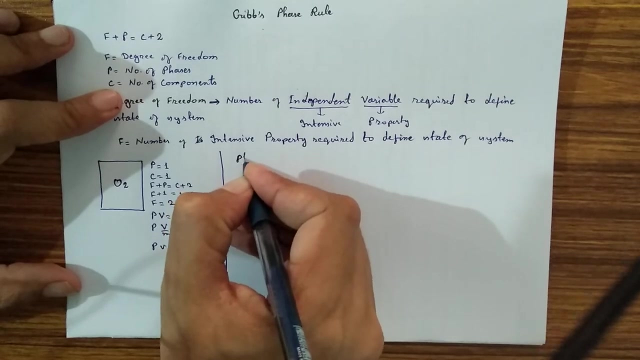 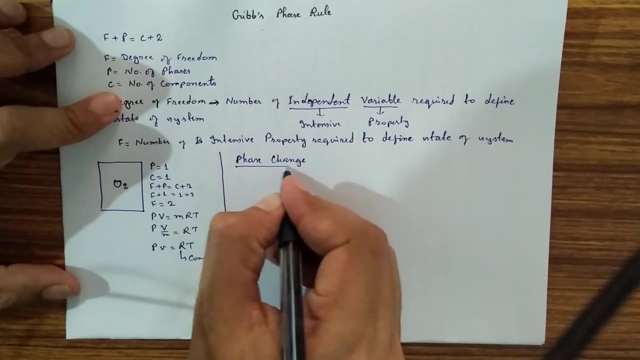 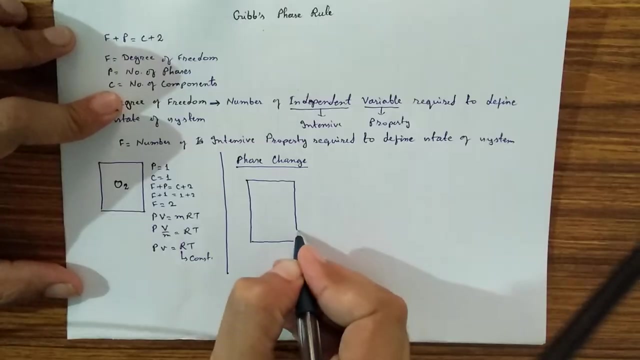 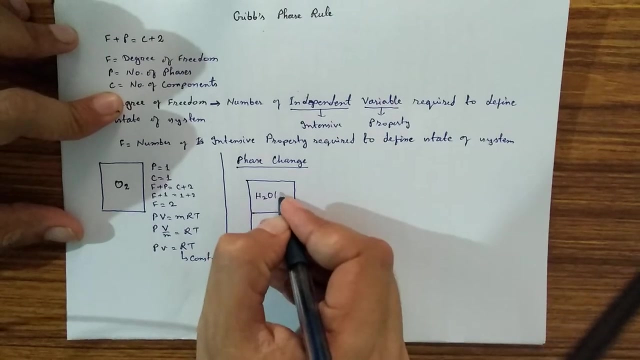 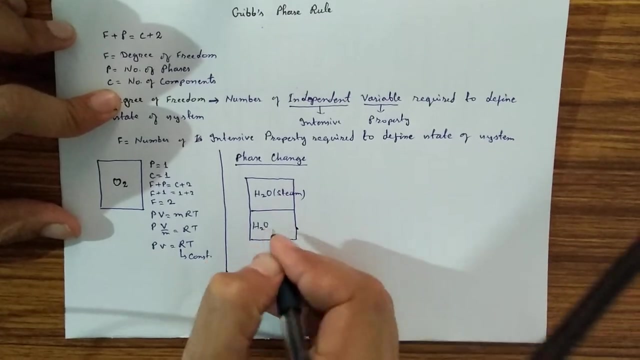 know this specific volume. if we know a specific volume, we will know pressure. and if you know a specific volume and temperature, we will know the pressure. so this is having 2 degree of freedom. we will take another example. let us see phase change for phase change: H2O steam and H2O liquid form, that is, water. 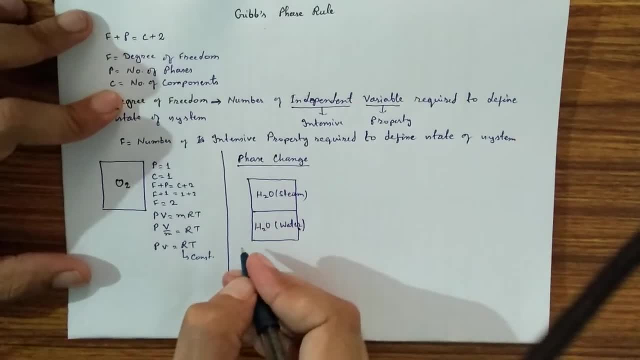 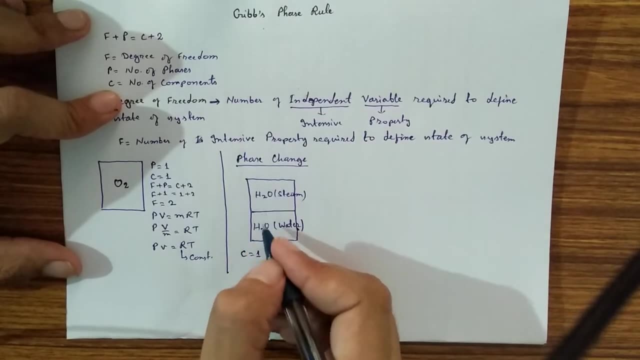 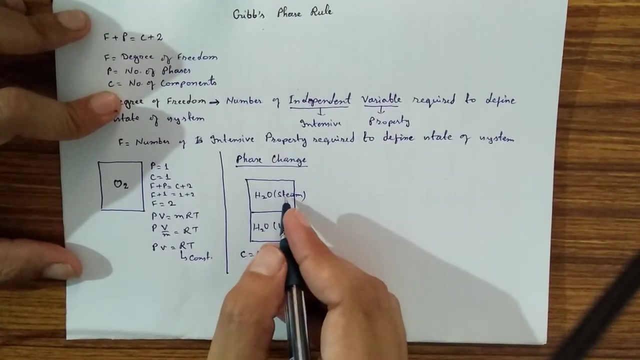 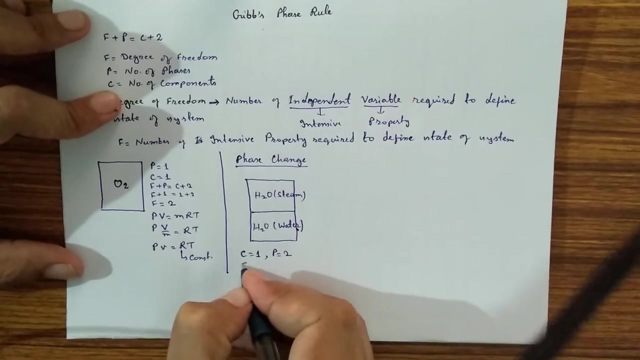 so here we have component, number of component as one, because this is only the forms of water. so only one component is here. so number of component is 1 and it is having two phases. one is in gaseous form and other is liquid form. so number of phases is 2, F plus P, equal. to C plus 2, that is F plus 2 equals to R2.. 1 component of water has two phases. the other is an air component of water that is a gas form and the other is liquid form. so phase is number of phases. 2 F plus P equals to C. 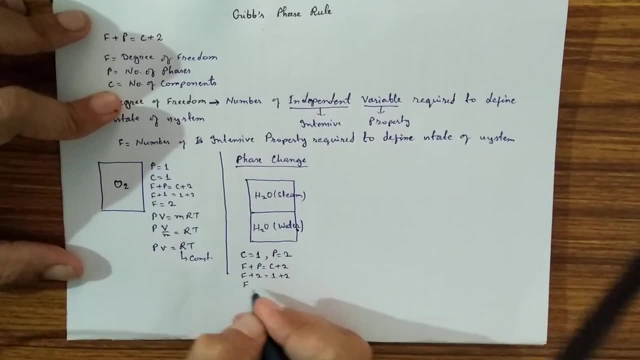 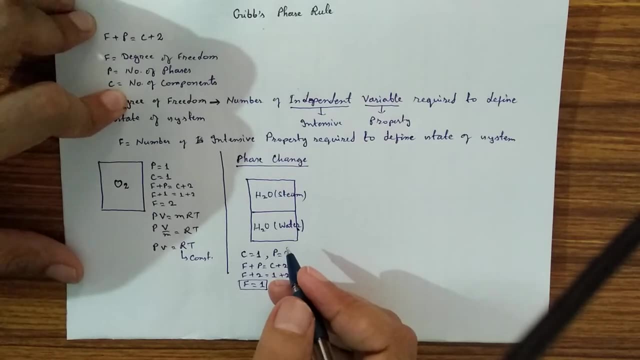 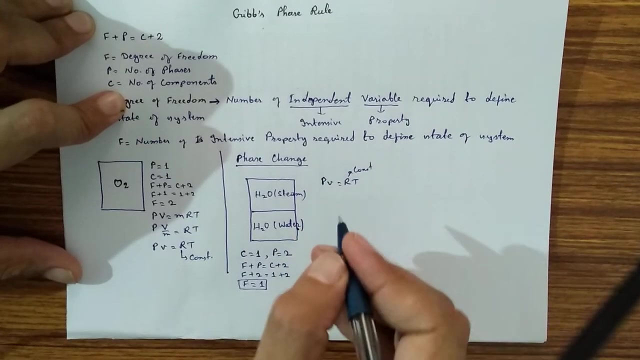 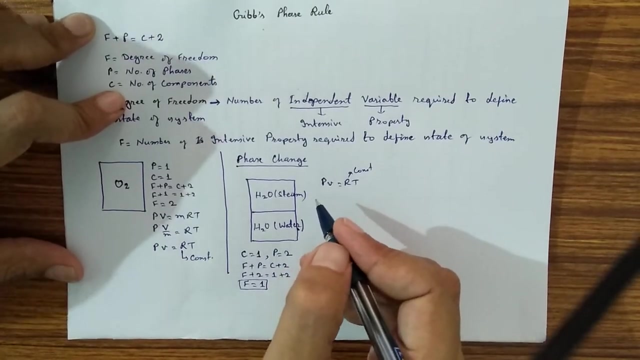 two equals to one plus two, that is f equals to one. so this is having degree of freedom one. during phase change, degree of freedom is one, pv equals to rt, r is constant and since it's having degree of freedom one, that is, if we vary one variable we will get the value of other variable. we know that in during phase change. 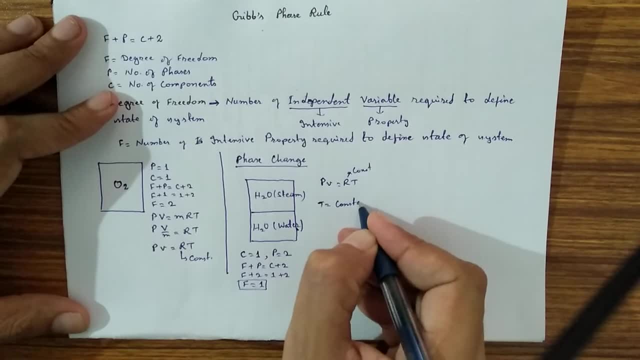 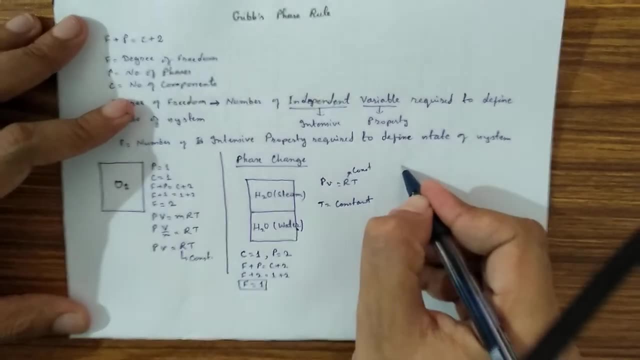 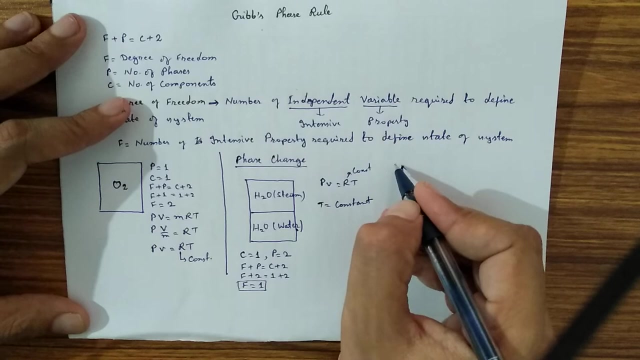 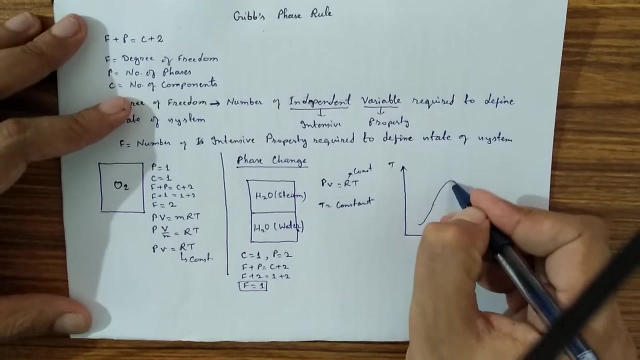 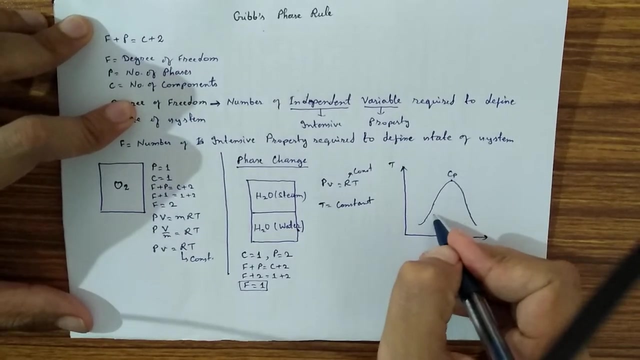 temperature remains constant. so since temperature is constant, there is only one degree of freedom. we can better understand this with the ts diagram. if we see ts diagram for phase change, this is critical point for state change. for example, we will have t s1 as constant for particle pressure. 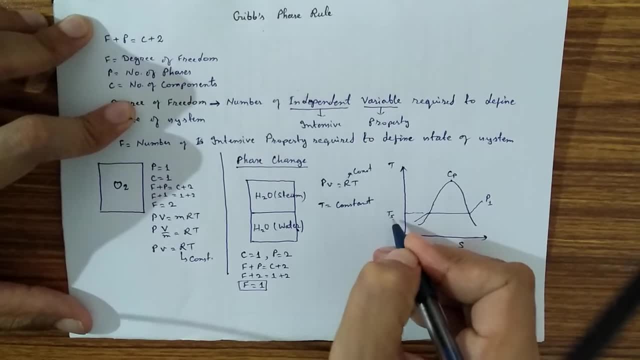 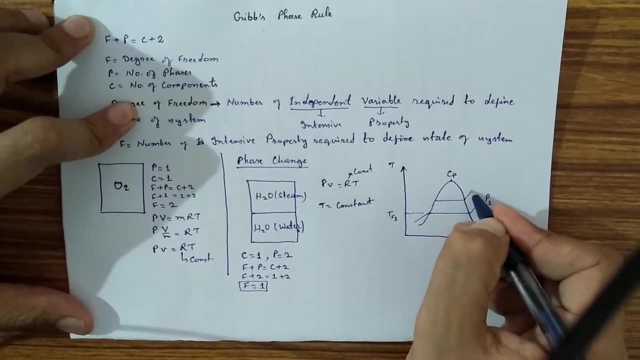 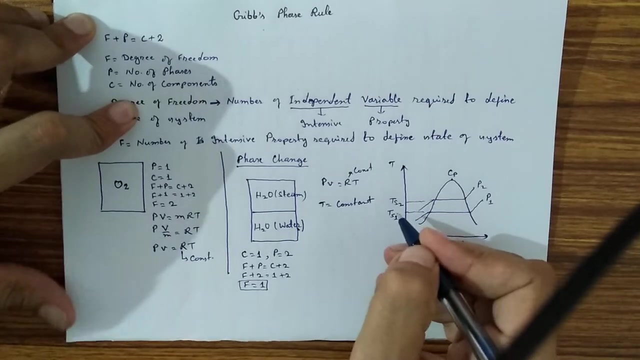 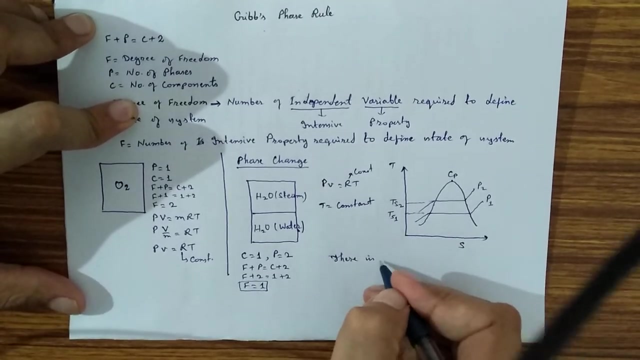 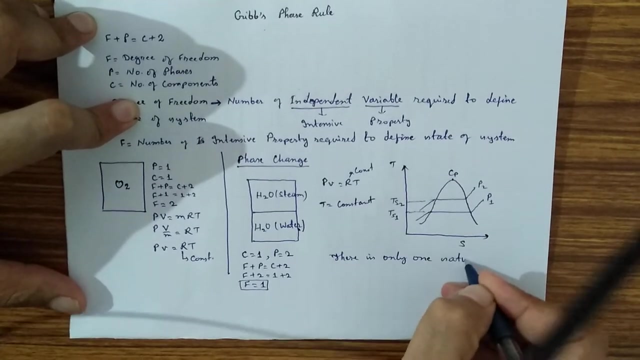 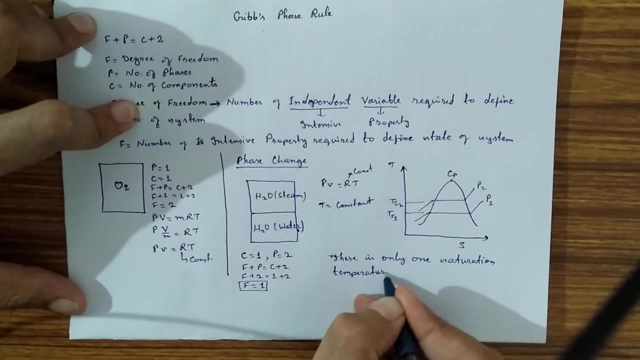 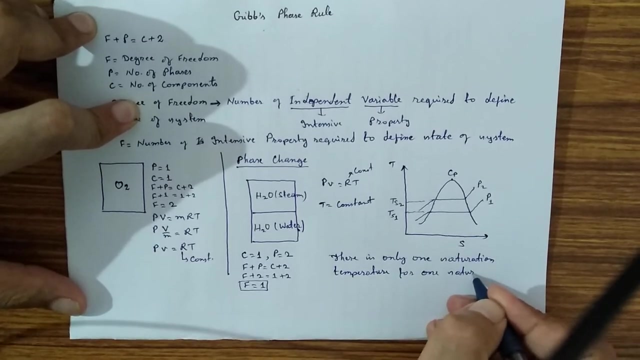 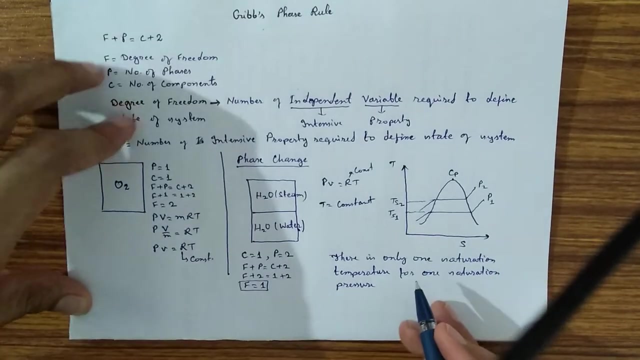 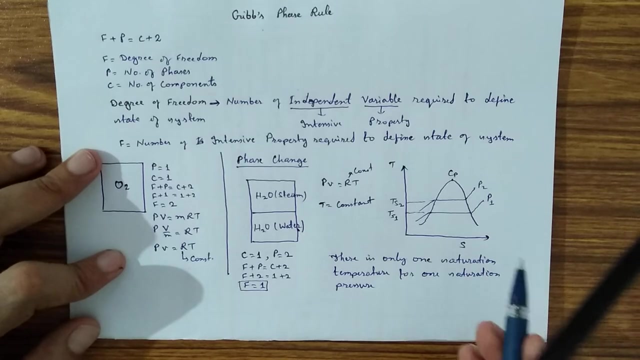 we will have a saturation temperature as once ts1. if we will change the pressure, p2 we will have and the saturation temperature. so there is only one saturation temperature. saturation temperature for one saturation pressure, so there is only one situation temperature corresponding to a saturation pressure. so for one situation pressure we will have one situation temperature and for 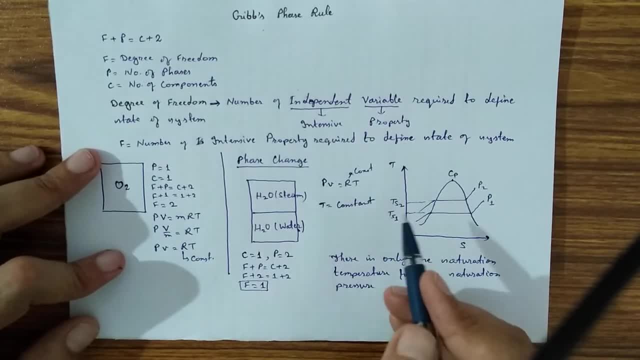 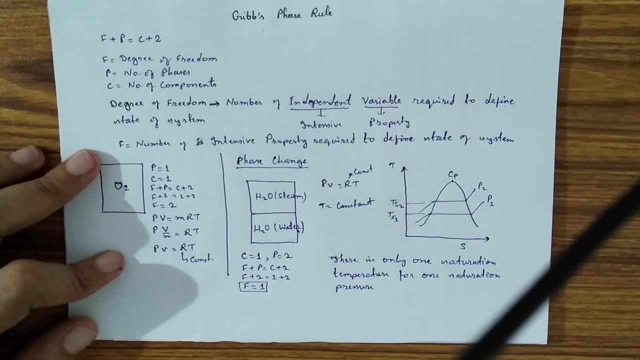 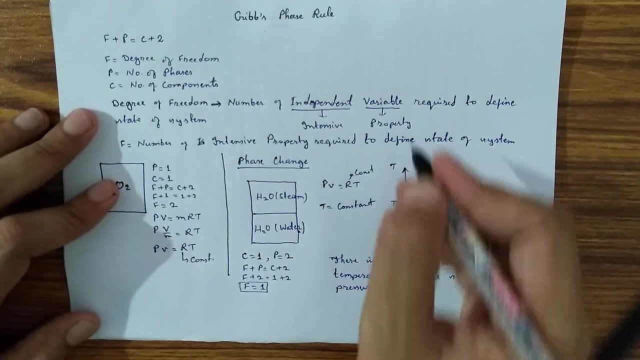 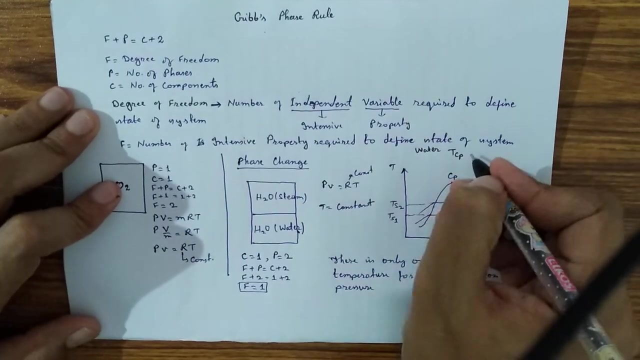 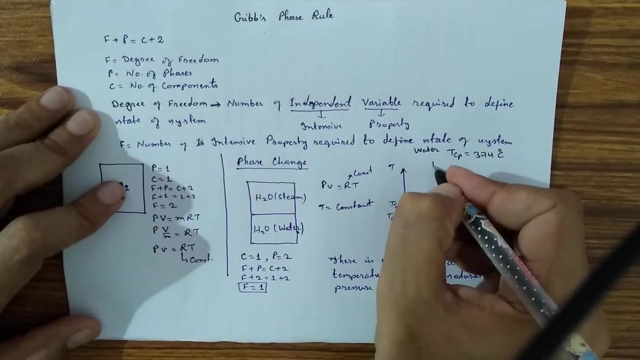 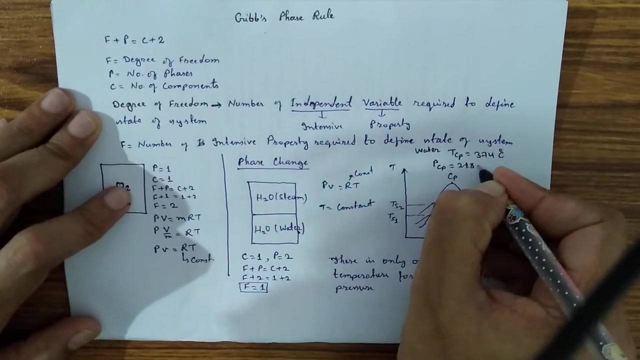 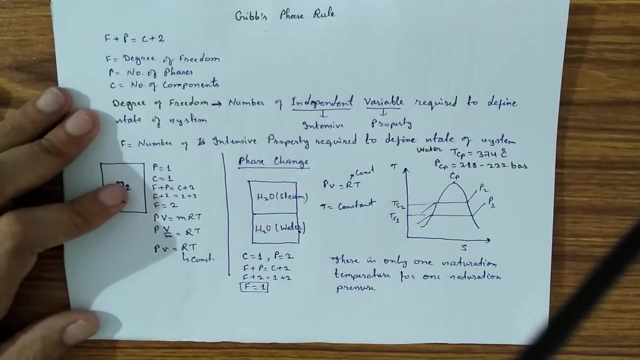 another situation. pressure, we will have another situation temperature, since the degree of freedom is one for phase change. for water temperature, critical point temperature is 374 degree centigrade and critical point pressure is two hundred eighteen bar, two sorry, 218 bar to 222 bar. now let's take another example. 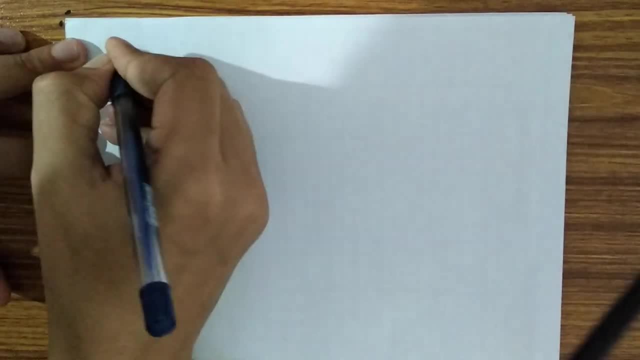 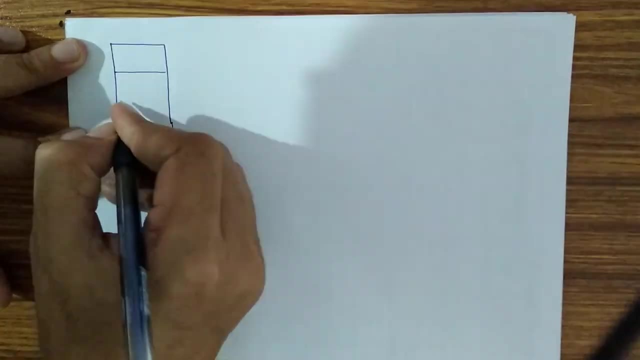 consider container having water in three forms: h2o in2007. water in three forms: H2O In sind Hayır. H2O Injes. h2o Injes. it is waterThat is discussed in 2aha Mirannen. it is water That is discussed in 2aha Mirannen. 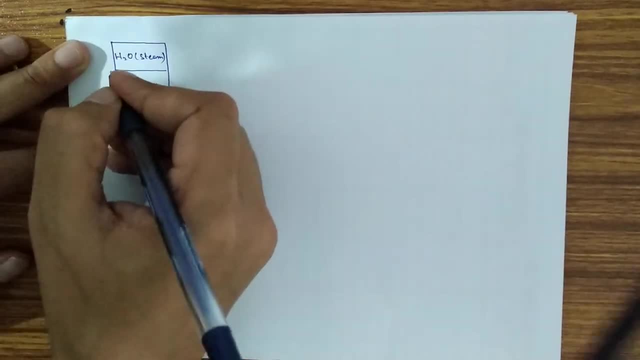 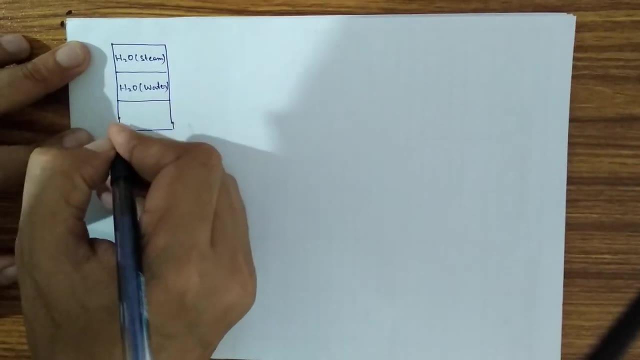 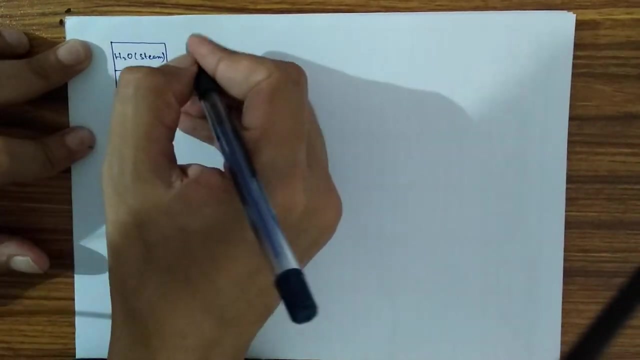 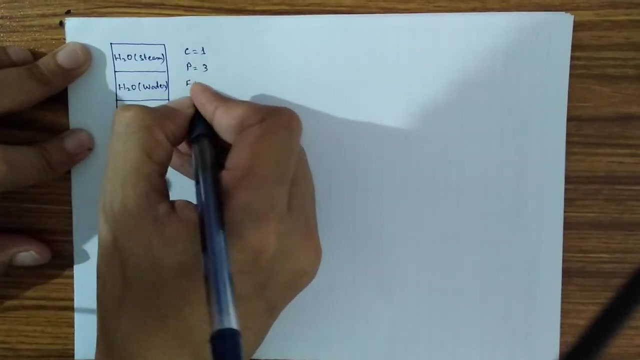 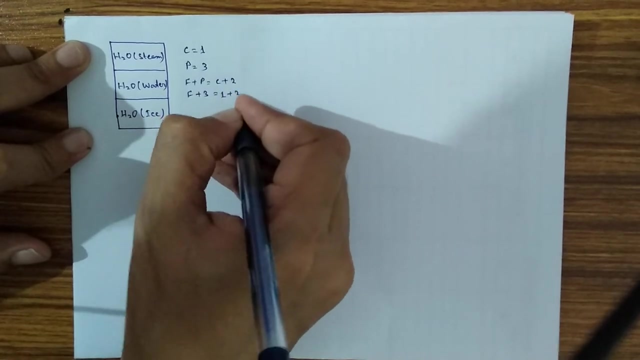 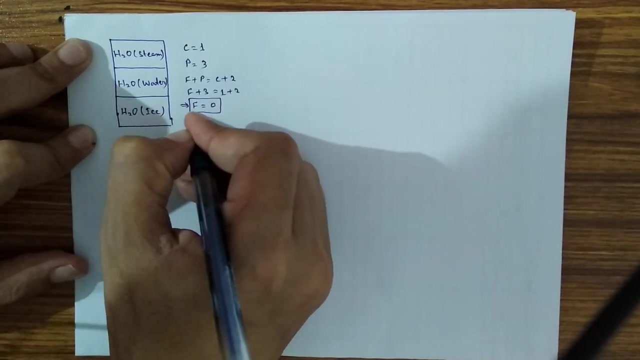 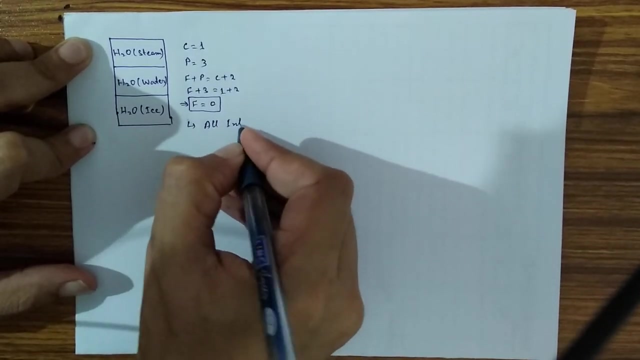 steam form- h2o, and water form- h2o, ice form. here number of component is one, number of phases is three. so F plus P equals to C plus 2. F plus 3 equals to 1 plus 2. that means degree of freedom equals to 0. that means all intensive. 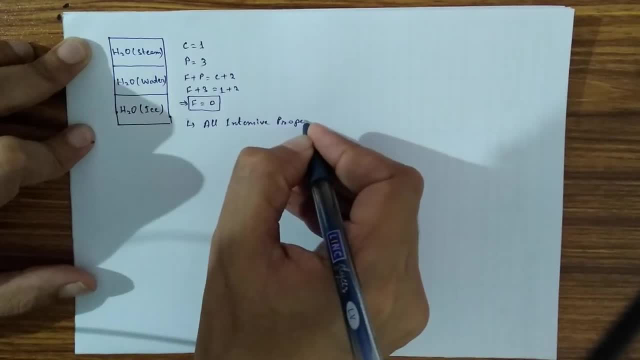 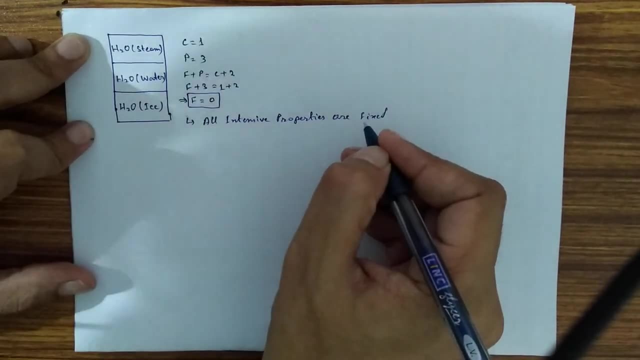 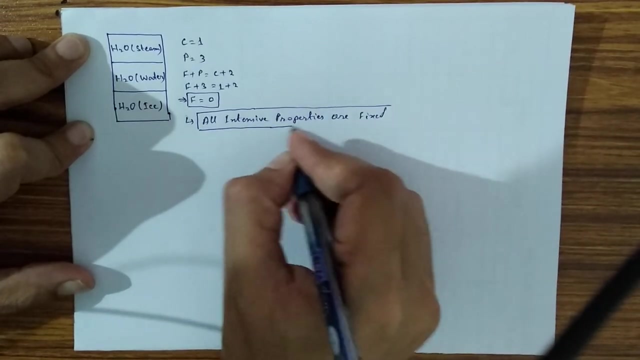 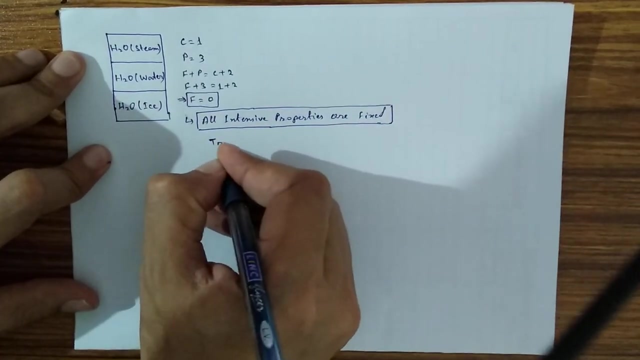 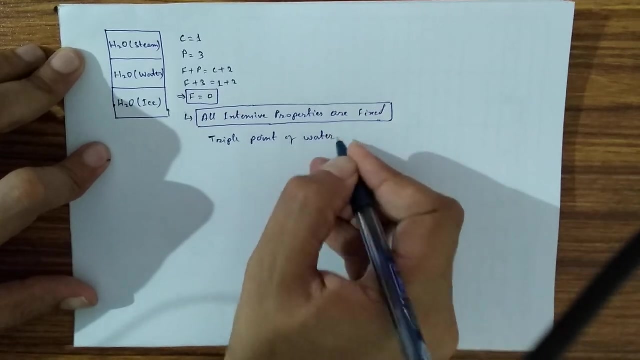 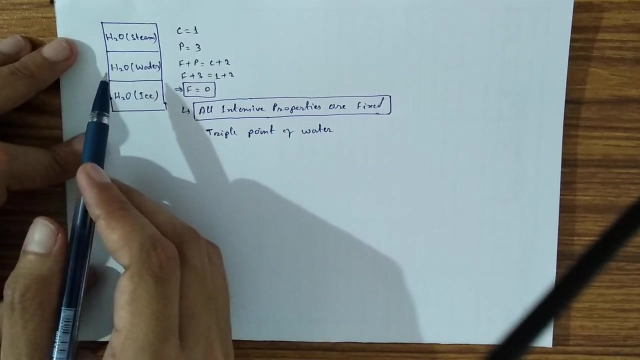 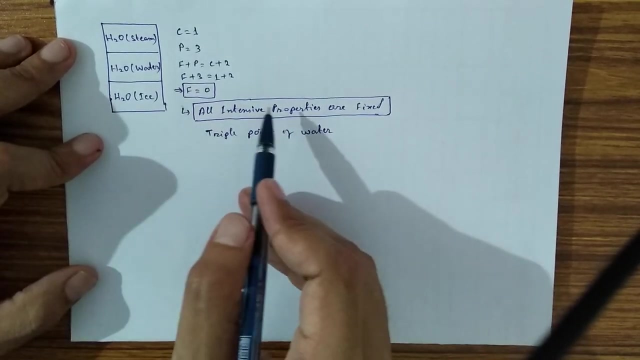 properties are fixed. all intensive properties are fixed. that is triple point of water. so this is the triple point of water. we are having steam, water, ice, all three phases present, so, due to which the degree of freedom is 0, that is, all intensive properties are fixed, since the degree of freedom is 0, so all intensive properties. are fixed, which is called triple point of water. we will see a triple point of water. temperature at triple point of water is 0.01 degree centigrade. it is fixed that is at triple point the watt temperature of water will be 0.01 degree.